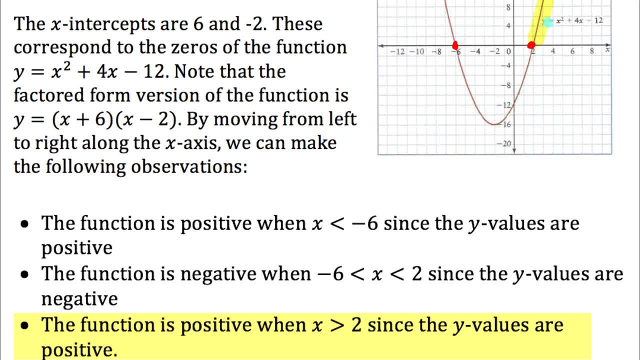 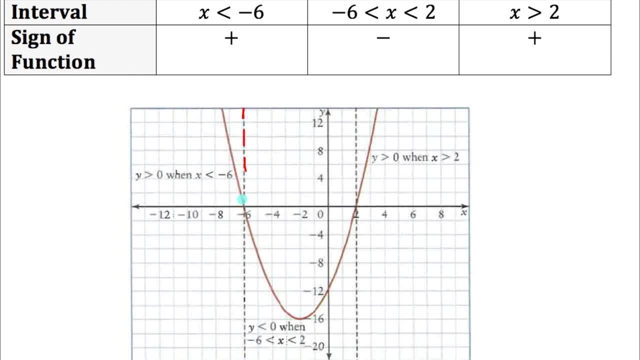 x-axis, All of the y values of the points on the function in that section are positive. So we say the function is positive when x is greater than 2. And I just have another graph here with vertical lines drawn through those x-intercepts So you can see that the x-intercepts are the places where 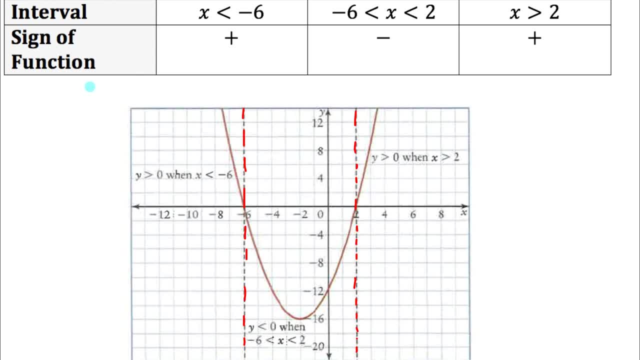 the function might change signs. If a function is above the x-axis, it's positive. If a function is below the x-axis, it's negative. So at the x-axis, the x-intercepts are the places where the function might change signs. So if we're commenting on one of the x-intercepts, we're 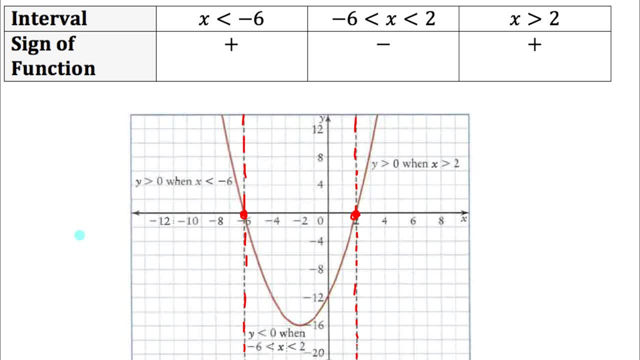 saying the function is positive or negative. we have to use those x-intercepts as dividing points that separate us into our intervals about where the function might be positive and where the function might be negative. In the first interval, which is described here, the function is positive. 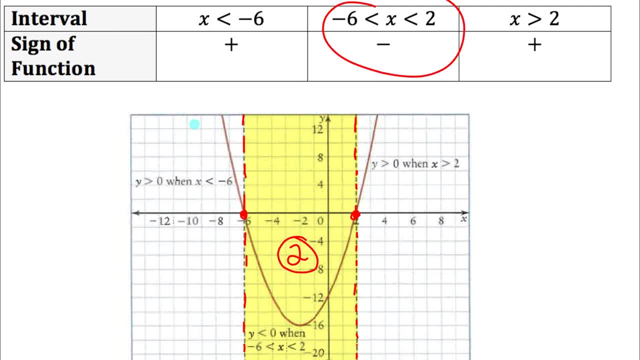 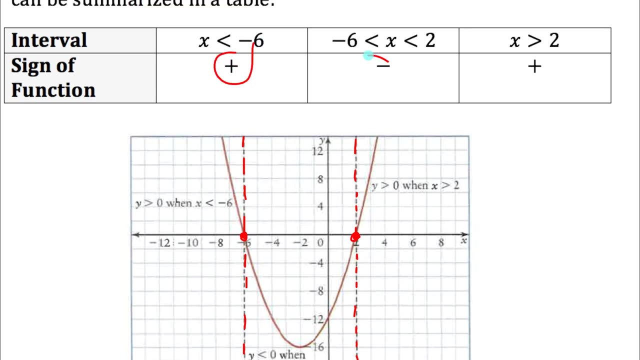 In the second interval, which is described here, the function is negative And in the third interval, which is described here, the function is positive. And remember, anytime I'm saying the function, I'm referring to its y values, I'm referring to the sign of the function based on its graph. but we could figure out the sign. 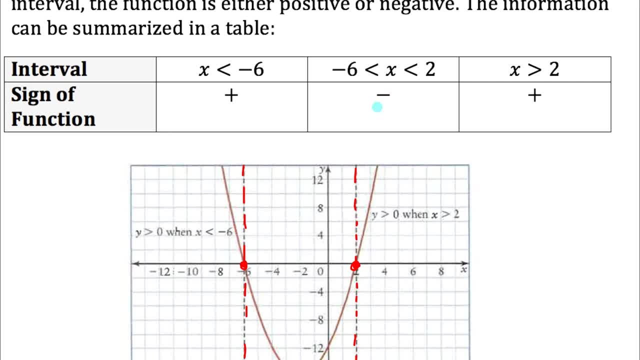 of the function from its equation as well. How could I tell from the equation that between negative 6 and 2, the function is negative? Well, you would just pick a test point. plug it into the equation. So we pick any test point within that interval. so how about an x-value of zero? plug it into the 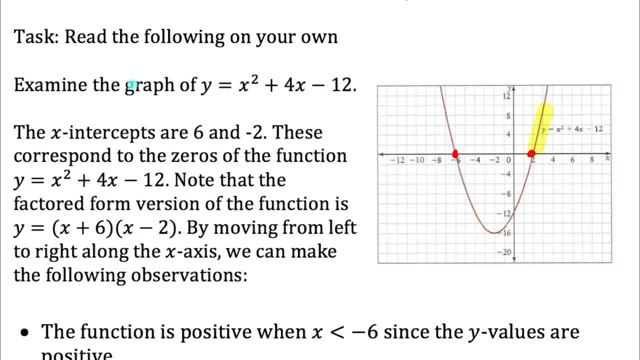 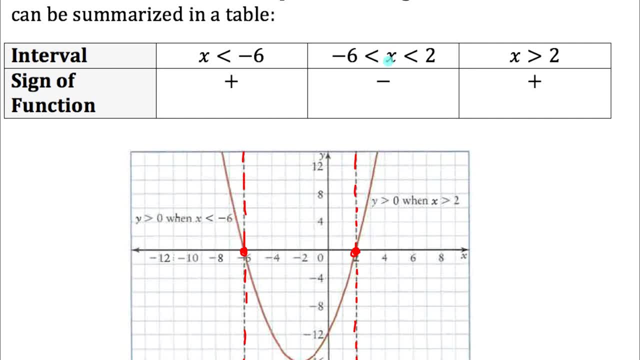 equation and we would get negative 12.. We figure out the function is negative within that interval And I know that within that entire interval it's going to be the same sign as any of the points because there are no x-intercepts within that interval where it might change signs. We know 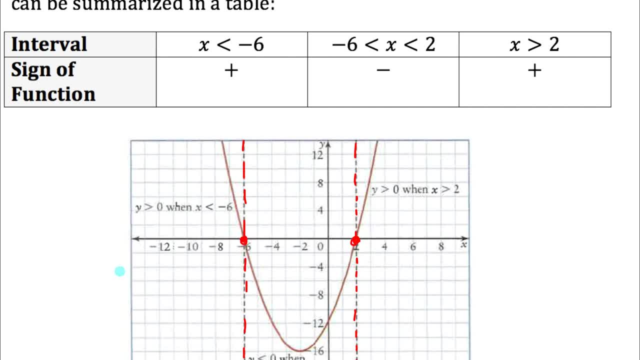 it's only going to change signs around the x-intercepts, and this is true for polynomial functions because they don't have any asymptotes. so the graph isn't going to do any weird jumping around. They're all going to be continuous functions that will only change signs at x-intercepts. 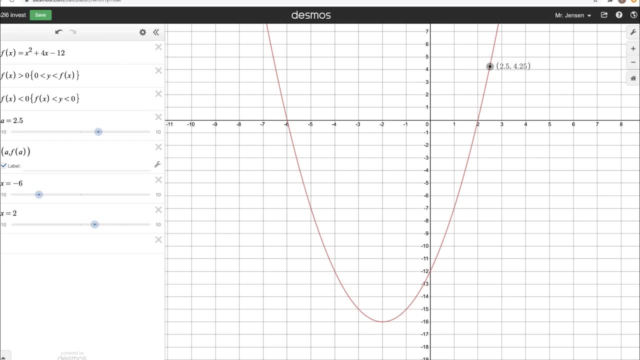 Just to make sure you fully understand this, I have this function graphed in Desmos as well. I'm going to draw the vertical lines through the x-intercepts and then I have a point on the function that I can move around. and while I'm moving this point, just pay attention to the y. 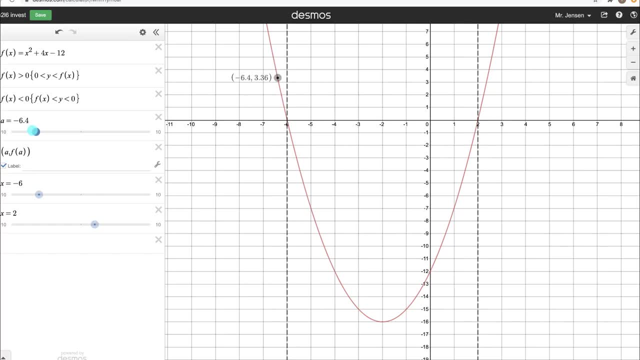 values of the point. So as I move this point, notice when is the function positive? Well, for any x value less than negative 6, I get a y coordinate that's positive. or for any x value greater than 2, I have a y value that's positive. So let me shade in the positive section of the 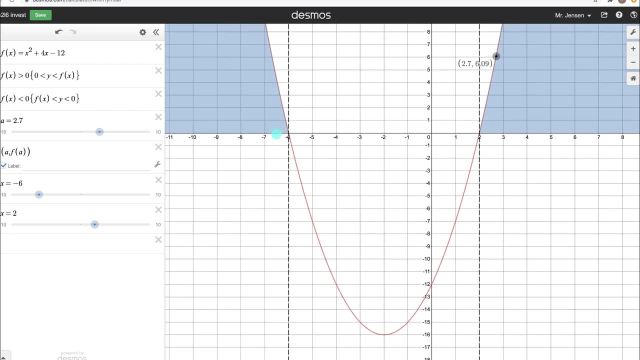 function. The function's positive when x is less than negative 6 or greater than 2.. When is the function negative? When is it below the y-axis? Well, for any x value between negative 6 and 2, look at the y coordinate of any of these points. They're all negative. so let me shade in that. 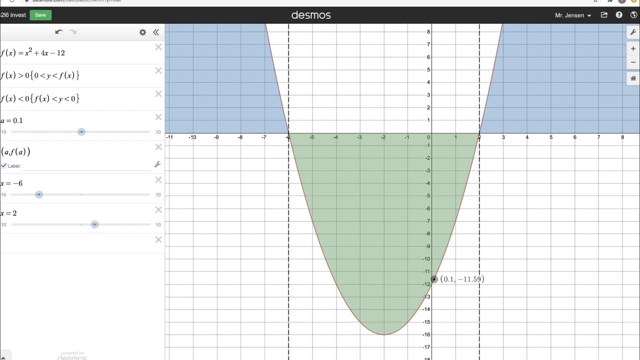 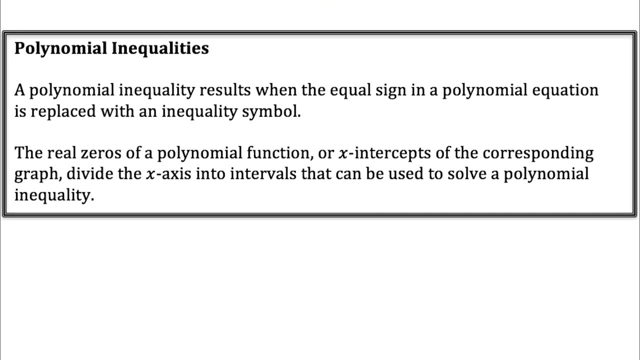 section of the graph. So the function is below the x-axis. it's negative for x values between negative 6 and 2.. So now that you understand how to describe when a function is positive or negative, we can actually go ahead and solve some polynomial inequalities. And what's an? 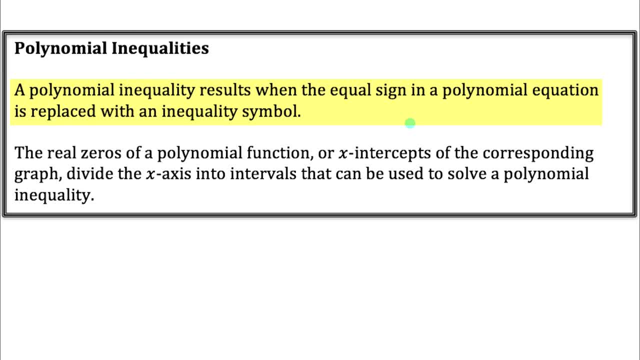 inequality. A polynomial inequality results when the equal sign of a polynomial equation is replaced by the equal sign of a polynomial equation, So when the equal sign of a polynomial equation is replaced with an inequality symbol, so like a less than or a greater than symbol. 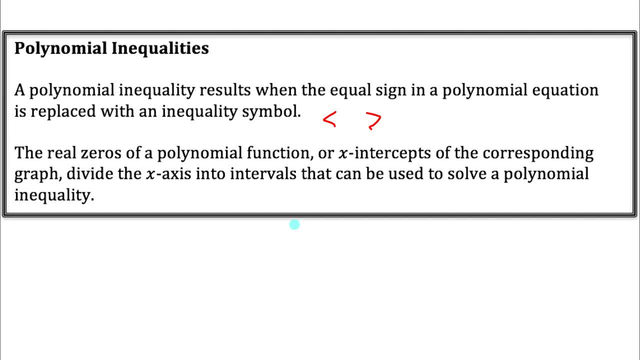 And we're often going to be solving for when is it less than or greater than 0, which is why we need to know when is a function positive or negative. The second part here says the real zeros of a polynomial function, or x-intercepts of the graph, divide the x-axis into intervals. 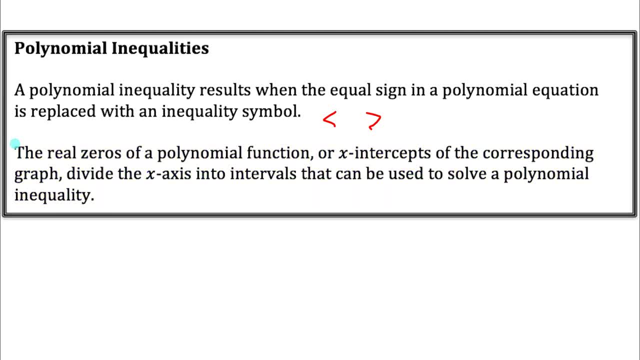 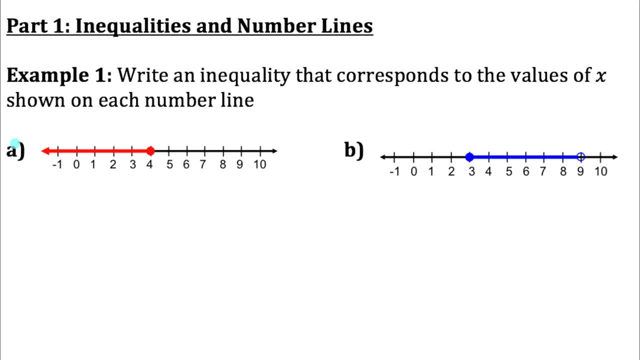 that can be used to solve a polynomial inequality. So the x-intercepts are going to be very important for us when solving polynomial inequalities. Before we jump into solving them, let's make sure you understand how to write intervals in a polynomial. So let's go ahead and solve a polynomial inequality. 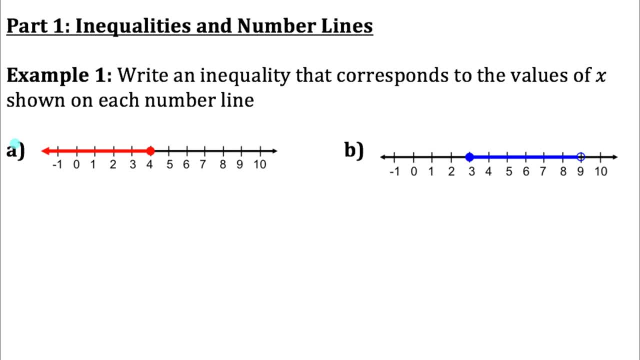 Let's first write the intervals of x-values both with inequality signs and an interval notation with round and square brackets. So example 1 says: write an inequality that corresponds to the values of x shown on each number line. Well, for part the number line looks. 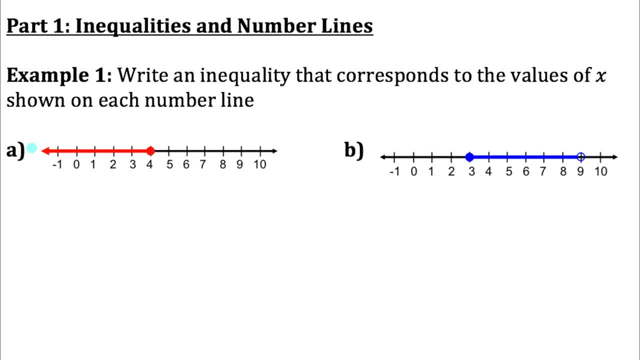 like it's describing x values at 4 and everything less than 4.. So I would say x less than or equal to 4.. That's as an inequality In interval notation. I would say x is an element of numbers which is an interval of x. So now I would write an interval notation with x values at 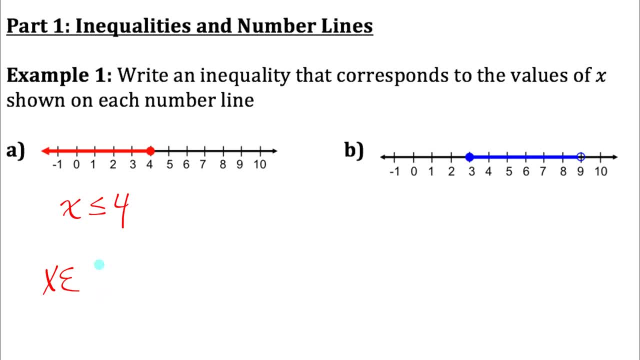 4. And to write that, I would write a linear algebra slash a linear algebra plus a integral of x. So this would be the order we would write an integral notation for. So we would write an interval numbers from negative infinity to 4.. Whenever you're writing the interval, you always do the 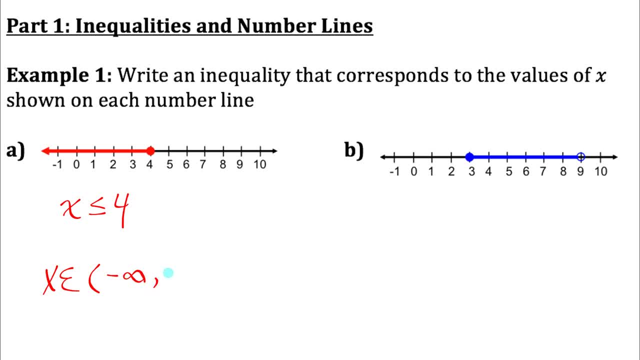 lower boundary comma, the upper boundary, so the min value comma, the max value, And 4 is included in this interval because the circle is filled in, so it would need a square bracket. Square bracket means the number is included in the interval. Part b: we're describing the interval from 3 to 9,. 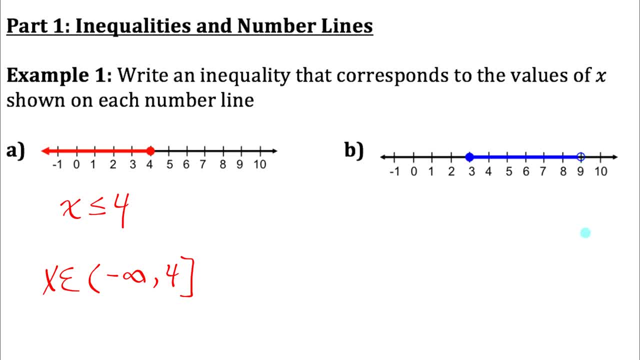 where it looks like 3 is included but 9 is not included, indicated by the open circle. So as an inequality, we would say x is between 3 and 9, and we want to include 3,, so I'll put an equal sign. 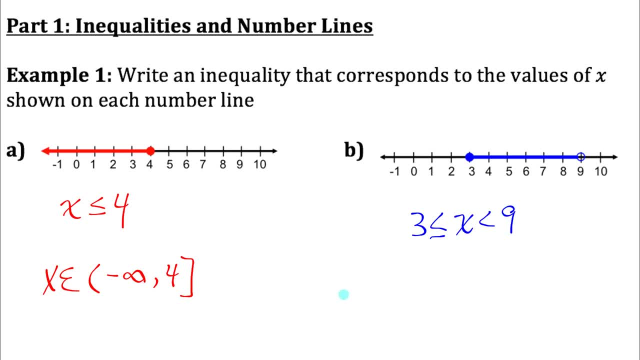 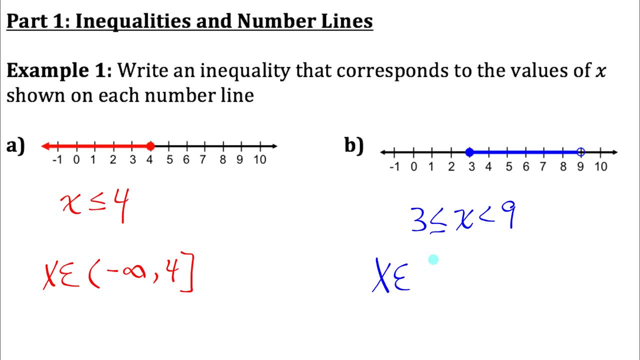 underneath that inequality, but not include 9, so no equal sign underneath that inequality As an interval, we could say x is an element within the interval from 3 to 9.. And notice: I put a square bracket at 3 because 3 is included and a round bracket at 9 because 9 is not included. 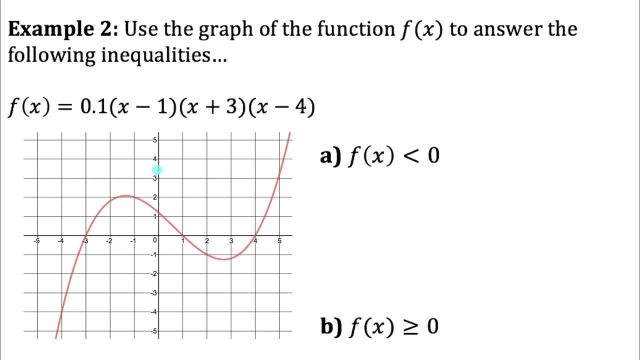 Let's slowly get to the end of this. Let's get into solving some polynomial inequalities. here This one: I'm giving you the factored form version of the equation and its graph Once we get to the end of the lesson you're just going to be. 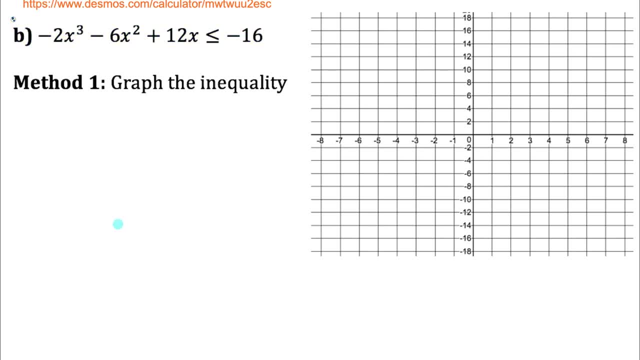 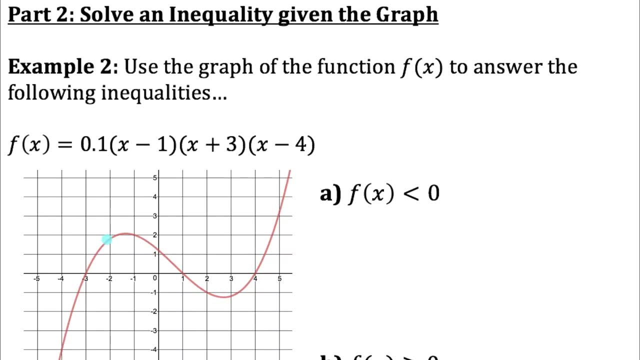 given the standard form version of the equation and not the graph, and we're going to have to generate the factored form version and its graph and use that to solve the inequality. But let's start by me giving you those things. Let's figure out: when is f at x, when is the? 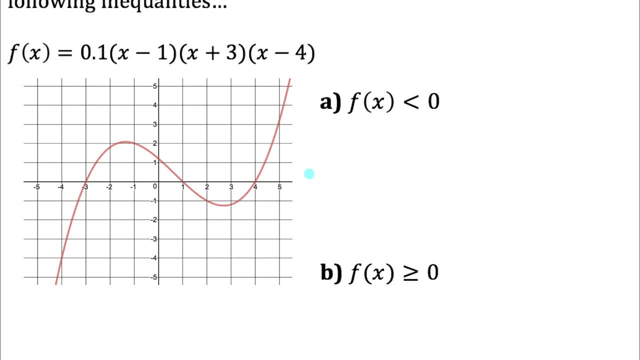 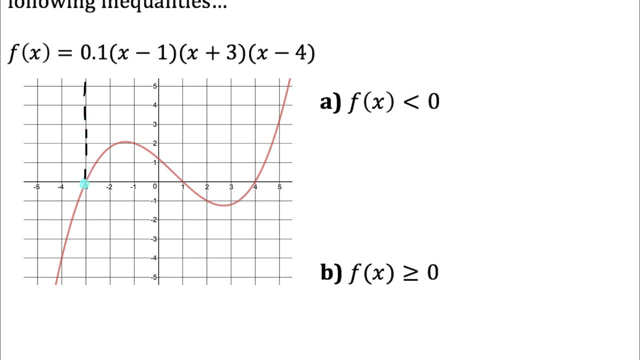 It may help if I draw the vertical lines through the x-intercepts. The x-intercepts are at negative 3,, 1, and 4.. That's going to divide the function into the intervals about where the function might switch between being positive and negative. So we're wondering: when is it less than 0?? 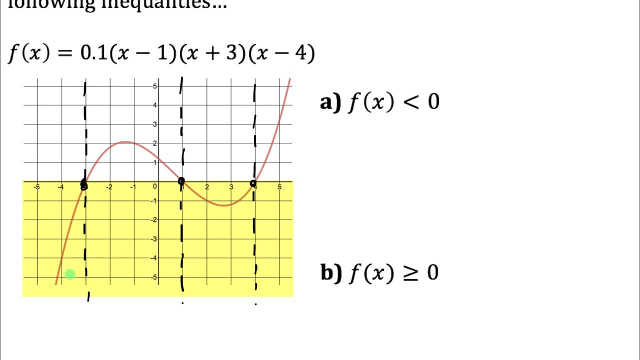 Well, the function is less than 0 when it's below the x-axis. Well, the function is below the x-axis right here and right here. So let me just shade in those two intervals. So in that interval and this interval the function is negative. So let's describe the. 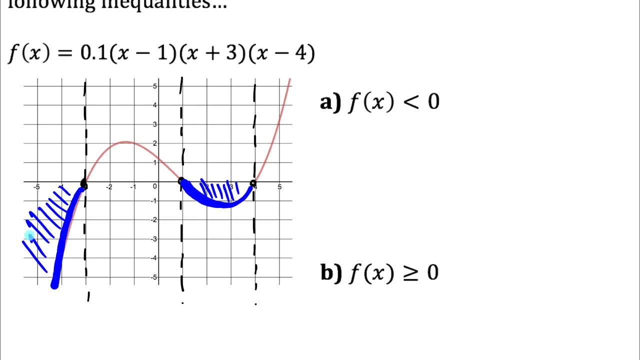 x values of those intervals. So this first interval that I shaded in here, it would be x values less than negative 3.. So we could say x less than negative 3.. And the next interval where it's below the x-axis, where the function's negative is between 1 and 4.. So we could say: 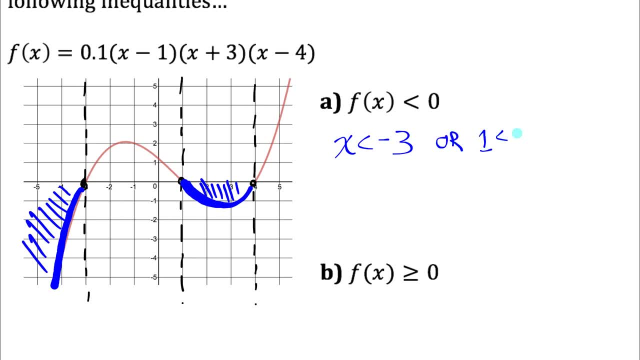 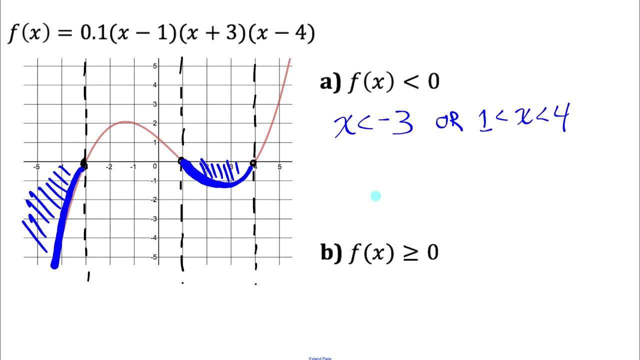 or when x is between 1 and 4.. Those are the two intervals where the function is negative. So the function is negative if x is less than negative 3, or if it's between 1 and 4.. If we want to write this in interval notation we'd say x is an element of numbers. 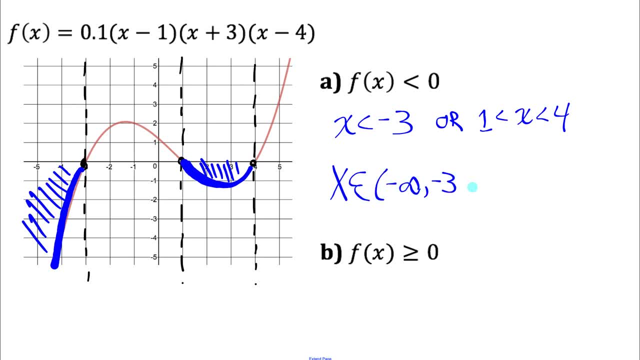 from negative infinity to negative 3, or from 1 to 4.. So we could say: or when x is between 1 and 4. And the next interval where it's below the x-axis. there are round brackets on each of those intervals and that's because we're just interested. 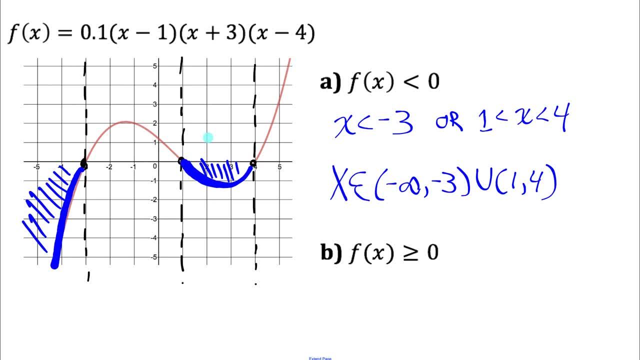 when is it less than zero? Not when is it less than or equal to just less than Part b says: when is the function greater than or equal to zero? So when is it above the x-axis? Well, the function is positive here and also here. So in this interval and also this interval. So let's. 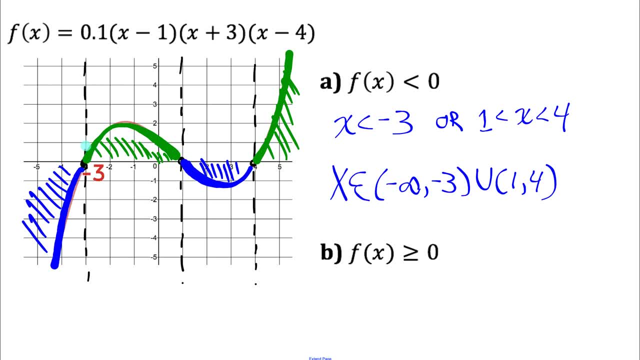 describe those two intervals. It would be from x values from negative three to one. and remember, at negative three and one the function is zero and we want to know when is the function greater than or equal to zero? So we want to include negative three and one in our answers. So we 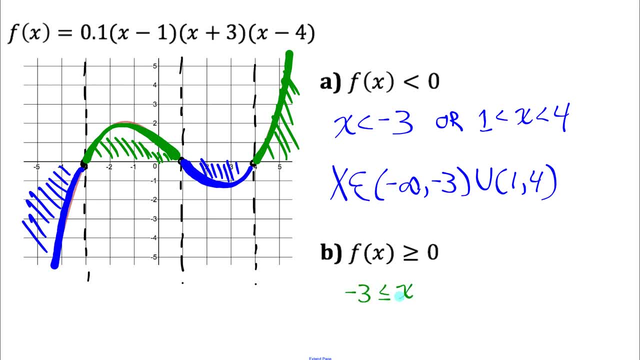 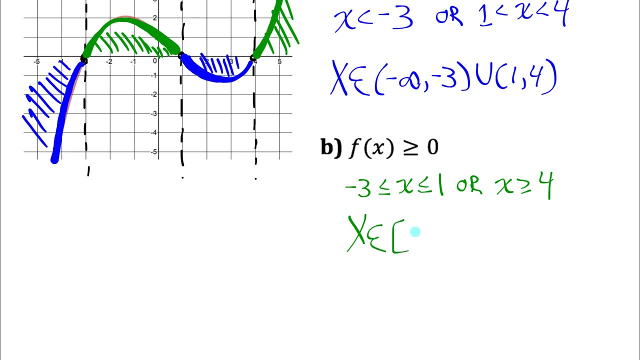 would say when x is between negative three and one, including negative three and one, or when x is greater than or equal to four, because at four it's zero. so we want to include that in our answer. In interval notation we would say x is an element and then square brackets between negative three. 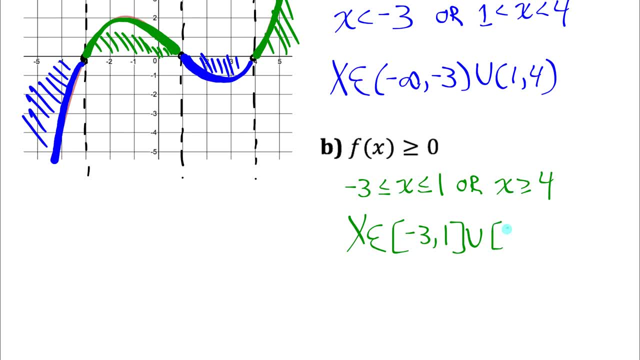 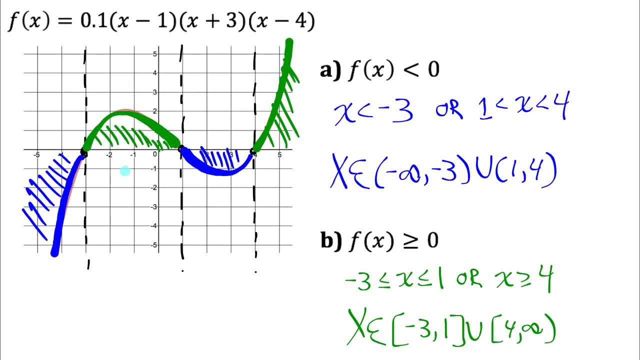 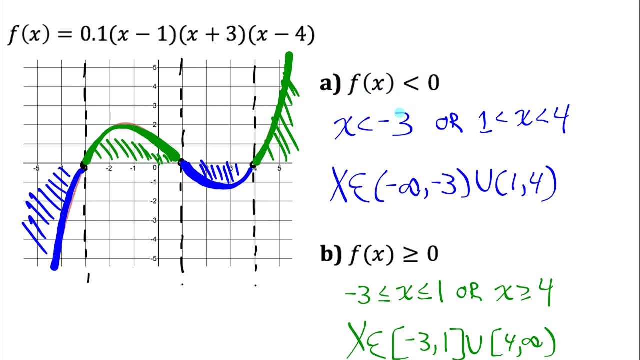 and one, or from four to infinity, and at infinity you always need a round bracket. And if you wanted to check if you did this properly- like we're saying that the function is negative when x is less than negative three, you could pick an x value less than negative three. like, let's say: 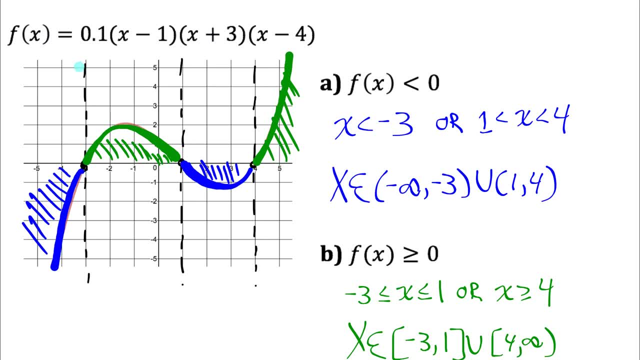 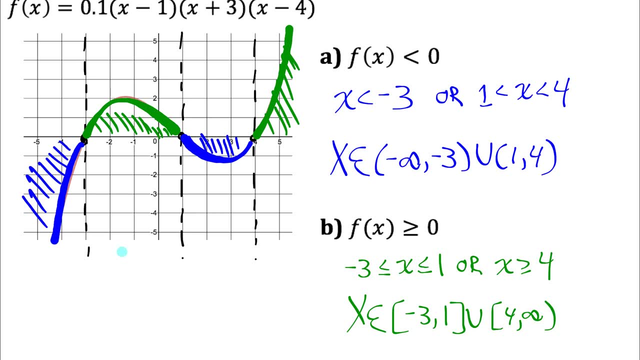 negative four. plug it into the equation and it should give you a negative answer, And that should be true for all the intervals that you've written. It should give you the proper answer. And when we solve them algebraically- that's what we're actually going to do- is pick. 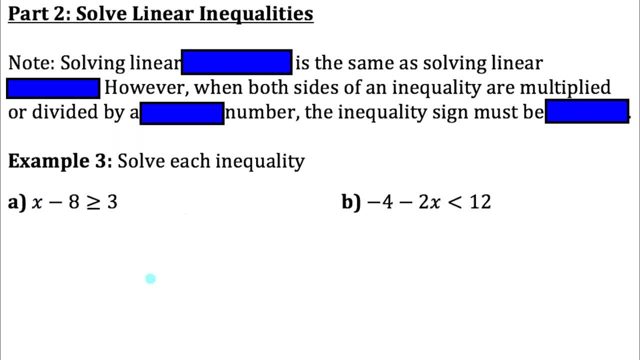 test points in each interval Before we get to the higher degree polynomial inequalities. I put in a couple linear inequalities for us to solve here, so degree one inequalities. If we're solving a linear inequality, it's actually the exact same as solving a linear equation, just with one rule. 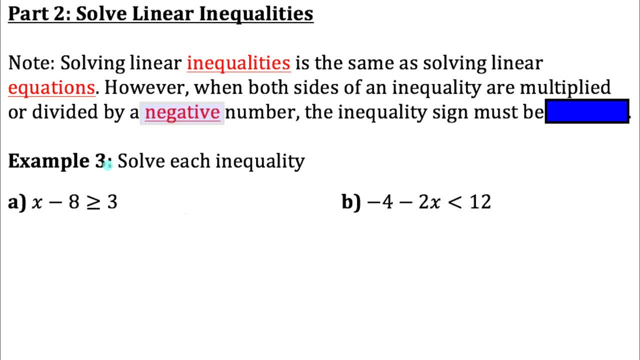 If you multiply or divide both sides by a negative number, you have to reverse the inequality sign. Other than that, you can solve them exactly like an equation. So this first one x minus eight is greater than or equal to three. If this inequality sign was an equal sign, well, I would just add eight to both sides. 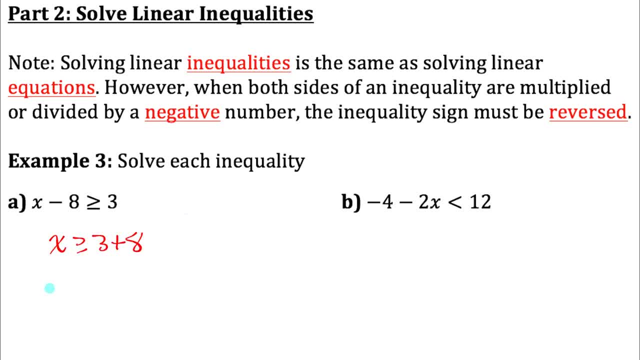 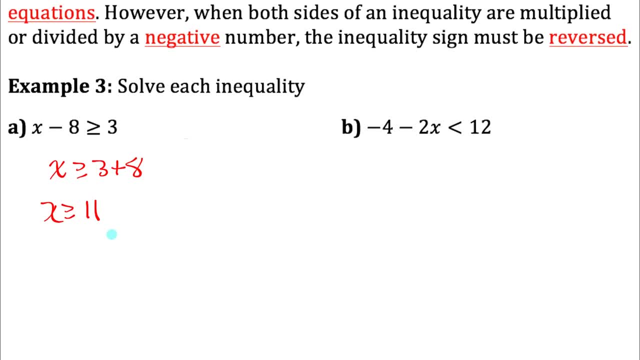 and I would get: x is greater than or equal to three plus eight. So x is greater than or equal to eleven, And that's it. That's all you have to do for this one. Solve it just like an equation. You can test it out if you want. Our answer says the original inequality is true for any x value. 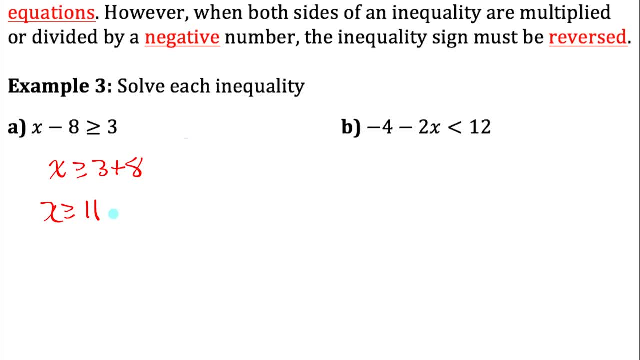 greater than or equal to eleven. So what's an x value greater than or equal to eleven? How about twelve? Test it out: Is twelve minus eight greater than or equal to three? Yeah, four is greater than or equal to three, So we have the correct answer. Part b: Let's solve this one like an equation. 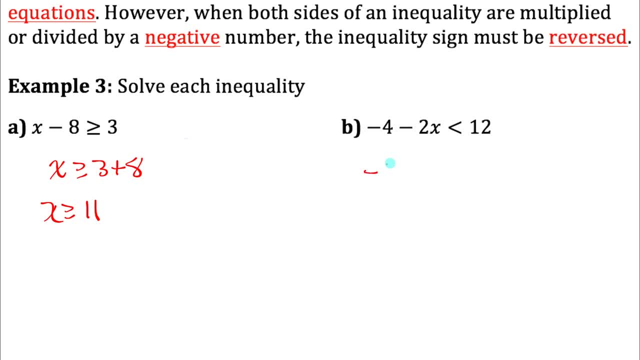 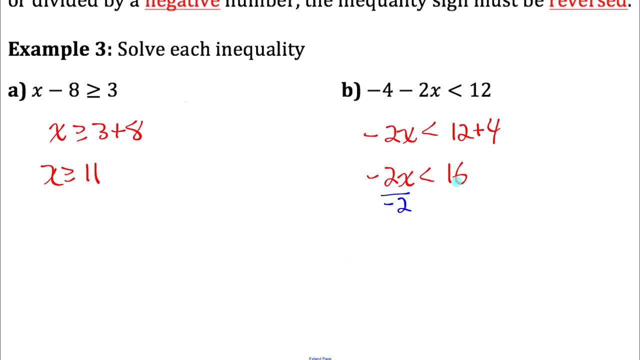 My first step would be to add four to both sides, So I would have: negative two x is less than twelve plus four, So negative two x is less than sixteen. And then the next thing I would do would be to divide both sides by negative two. And remember, if we look at the rule up here, when 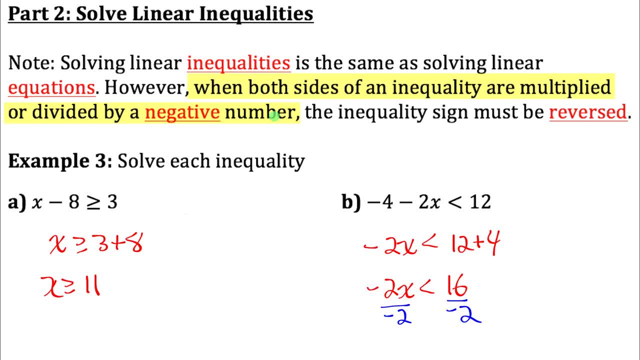 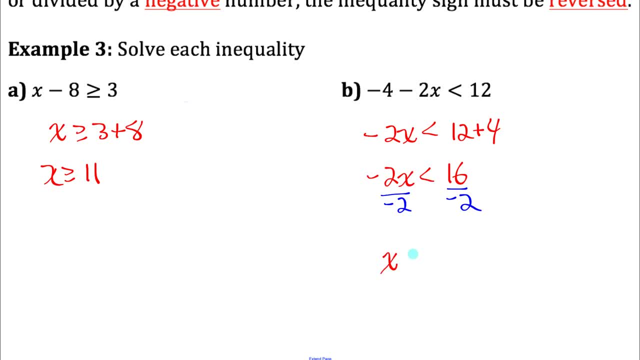 both sides of an inequality are multiplied or divided by a negative number, you have to reverse the inequality. So on my next line, I would have x, not less than negative eight. I have to reverse the inequality and it's going to be greater than negative eight. And let's test out this answer. 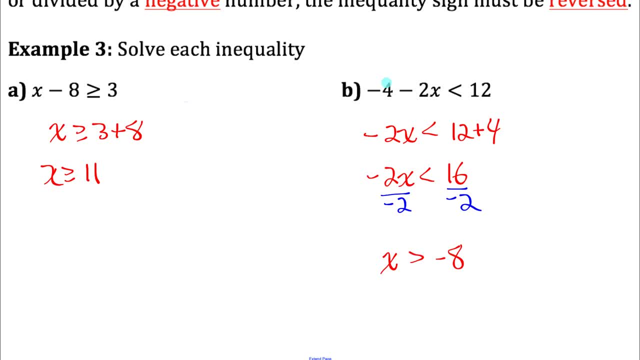 Apparently, if you pick an x value greater than negative eight, it makes the original inequality true. What's an x value bigger than negative eight? Well, how about zero? Plug in zero for x. negative four minus two times zero, That's just negative. four Is negative four less than twelve. 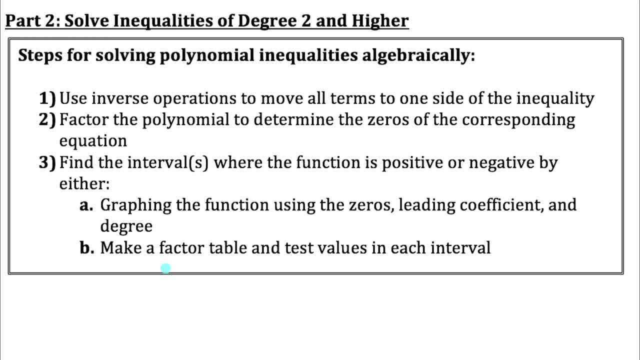 Yes, it is. So. solving linear inequalities is easy. Solve them just like equations, with that one extra rule. But if we have a degree two or higher polynomial inequality, there are two different ways we can solve it: Either graphically or by using a linear equation. Either graphically, 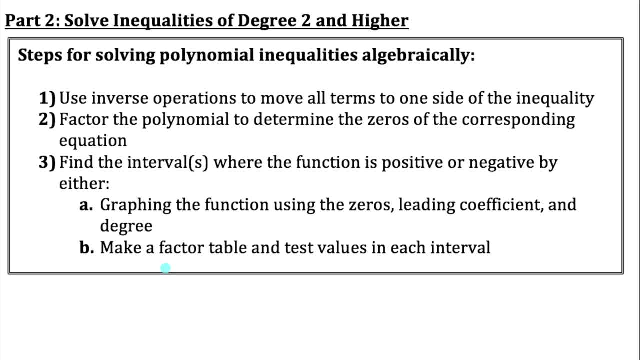 or by using a linear equation. Either graphically or by using a linear equation. Either graphically or algebraically, But in either of those ways the first couple steps are always the same. Start by doing inverse operations to move all terms to one side of the inequality. We always want one. 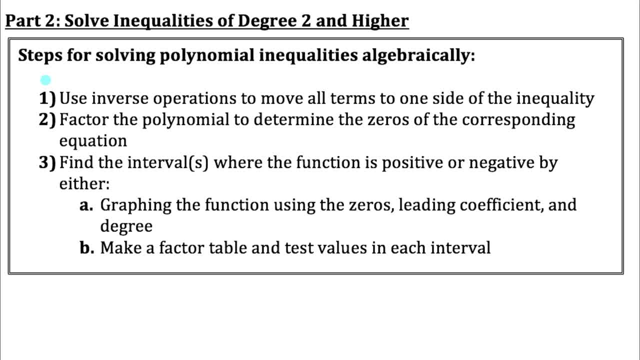 side of the inequality to just be zero. That way we're looking at when is the function either greater than or less than zero? so we can use the x-intercepts as the dividing points and check if the function is positive or negative. Step two: after we have everything on one side, we're going. 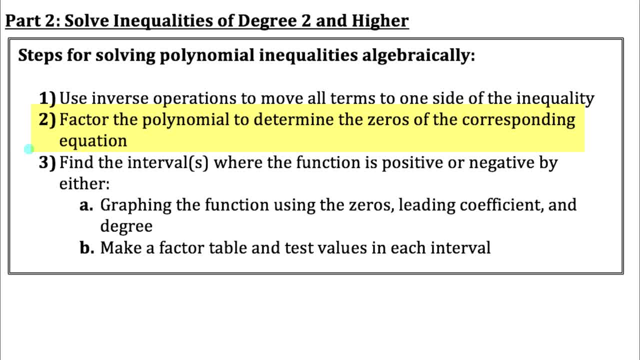 to get the polynomial into factored form and find its zeros, find its x-intercepts. After we have all the x-intercepts, we have two options. We can do a rough sketch of the graph using its zeros, leading coefficient and degree and then comment on where is the function positive or 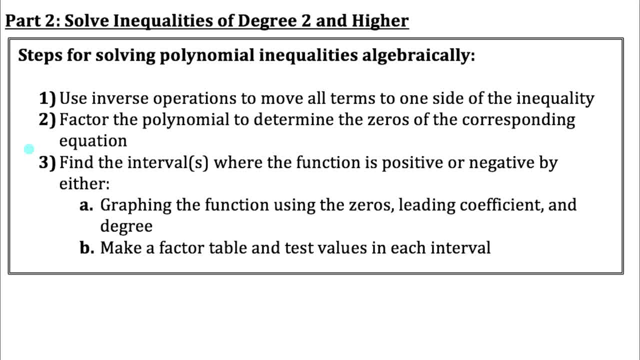 negative and that'll help us figure out the answer to our inequality. Or we could do it algebraically and make something called a factor table or sign chart and actually test values within each interval in the equation and get the equation to tell us whether the function is. 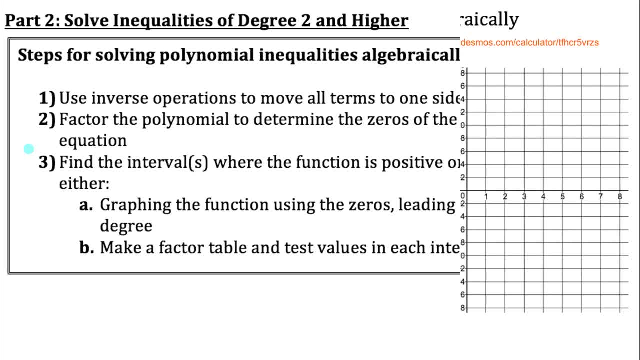 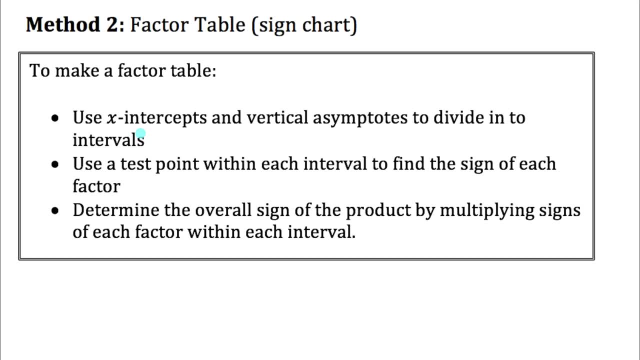 positive or negative within each interval. So I'll take you through both ways. So we're going to do three examples For each example. I'm going to take you through method one, where we solve it graphically, and method two, using a factor table. So part A it's a degree two, polynomial inequality. If I want to, 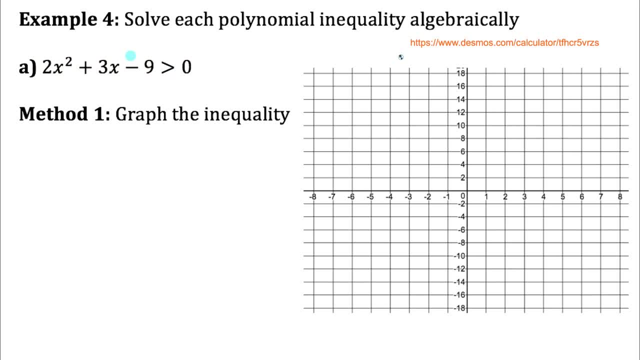 solve this one step. one is move everything to one side. It already is. All the terms are on the left. On the right I just have zero. So I'm interested in: when is this function greater than zero? So, graphically speaking, that would be: when is this function above the x-axis? When are its y-values? 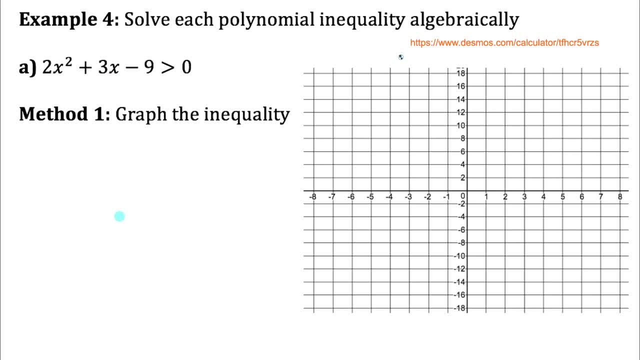 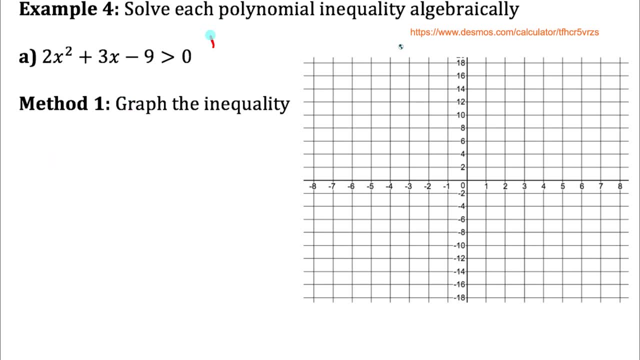 positive. So we need to start. if we're going to graph it, we need to know where are its x-intercepts. So let's get this into factored form. So I'd be looking for what numbers have a product of A times C, so a. 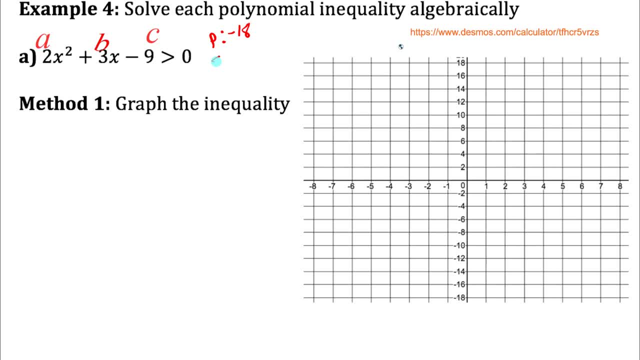 product of negative 18, and a sum of the b-value, a sum of 3.. Those numbers would be 6 and negative 3.. So I could split the middle term into 6x minus 3x and then factor this by grouping Common factor. 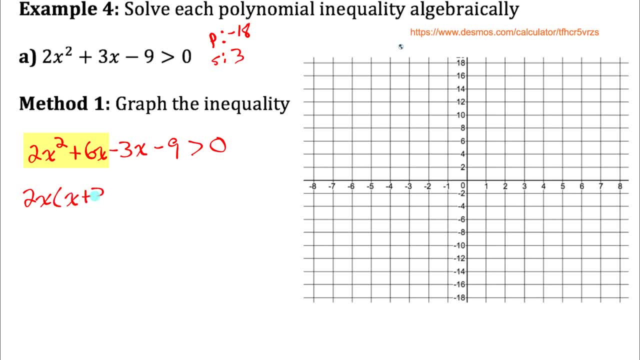 from the first two terms, I could take out a 2x and be left with x plus 3.. And from the last two terms, common factor, a negative 3 and get an x plus 3 again. Notice the common binomial We can common. 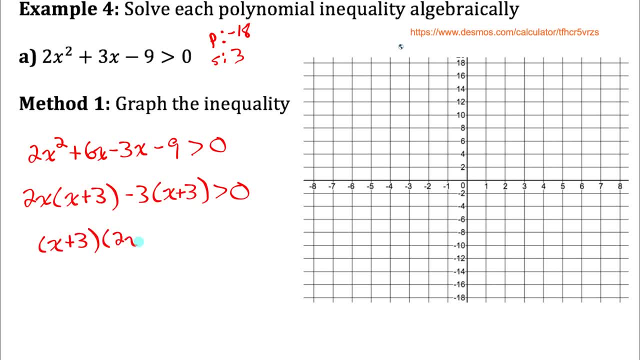 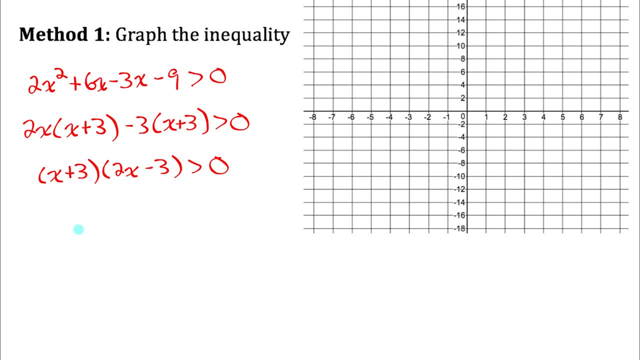 factor out that common binomial and have 2x minus 3 as the second factor. Okay, that's now in factored form. From the factored form inequality I could comment on. what are the x-intercepts? The x-intercepts: 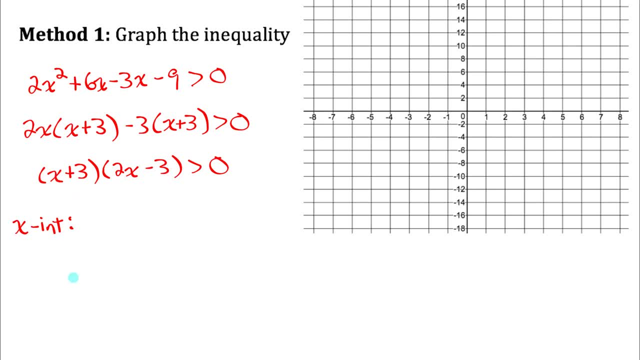 are the x-values that make it be zero. What would make this product be zero is if either the factors were zero. The first factor would be zero if x was negative 3, and the second factor would be zero if x was 3 over 2,, which is 1.5.. 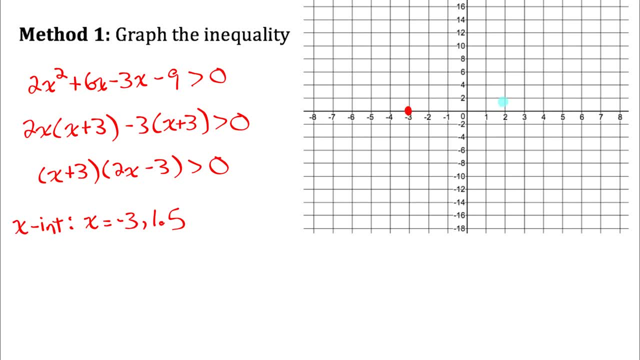 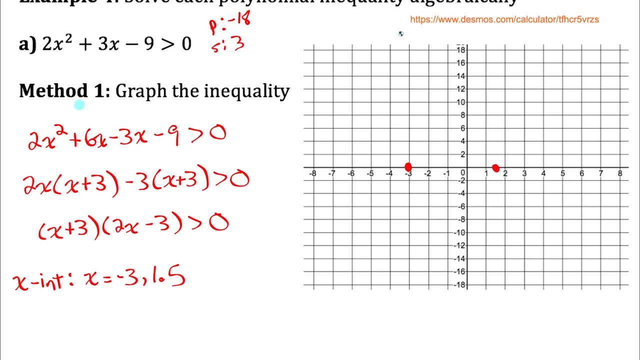 So I've listed the x-intercepts. They're at negative 3 and 1.5.. Now all I need to know is the general shape of this function. Well, it's a quadratic, so that's a parabola, And also I know. 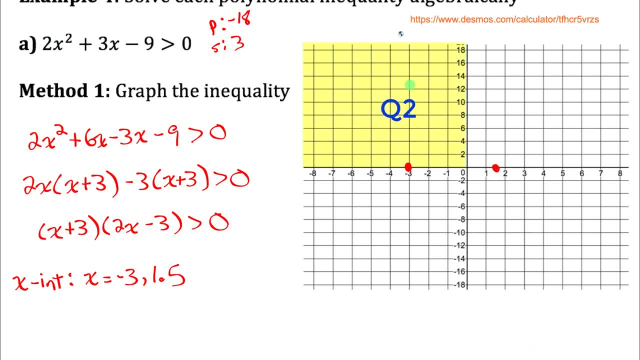 that it's even degree positive leading coefficient. so it has to go from quadrant 2 to quadrant 1.. I don't really care where the x-intercepts are, I just want to know where the x-intercepts are. I don't care where the vertex is. I don't care if the vertex is here or here or here, It doesn't. 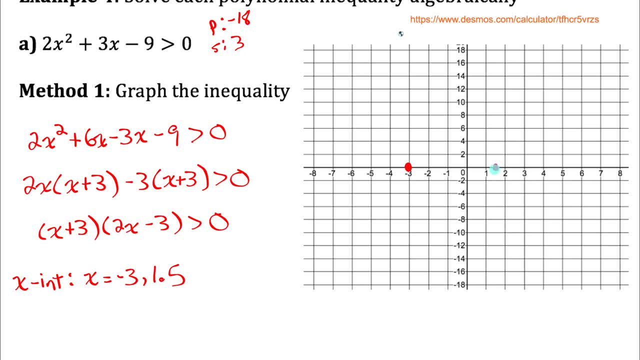 matter. I know it's going to be between those x-intercepts, but I don't care what the y-value is. I'm only interested in when is the function greater than zero? And if I do a rough sketch of this function using its n behavior, I'll be able to answer that inequality. And, like I said, 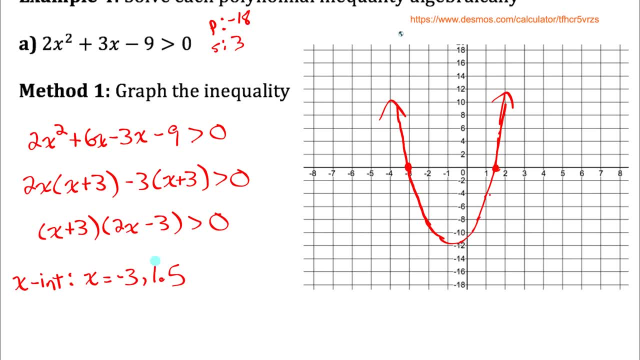 that vertex probably isn't in the right spot, but that's okay, I only care. when is this function positive? When is it above the x-axis? And if we look, the function is positive here and here. so I just have to describe those intervals. So the original question wants to know: when is the quadratic? 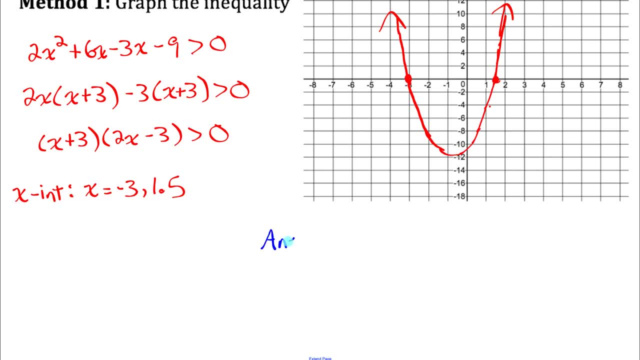 greater than zero. I'll write answer. The original polynomial is greater than zero in this interval, so when x is less than negative 3, or in this interval when x is bigger than 1.5,, so when x is greater than 1.5.. 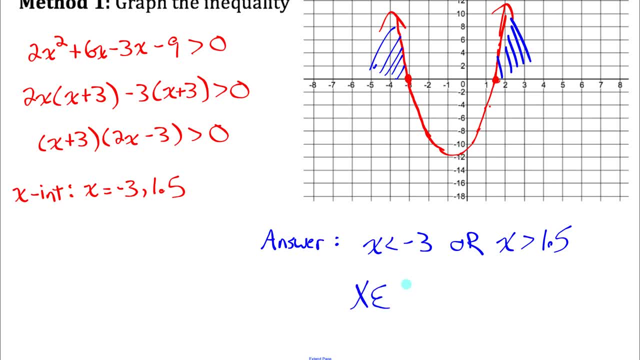 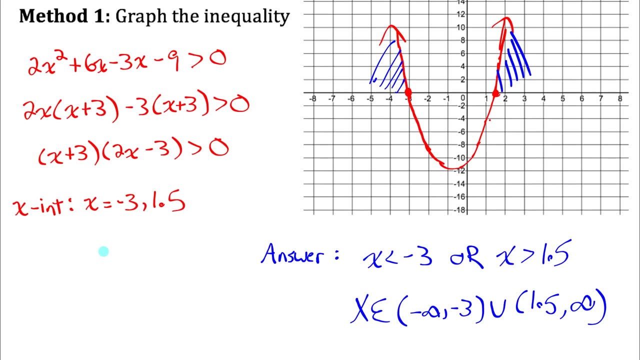 I could write that same answer in interval notation by saying: x is an element of numbers from negative infinity to negative 3, or from 1.5 to infinity. Those are two ways of stating the same intervals of x-values, And let me just show you on a graph that we have found the correct answers. 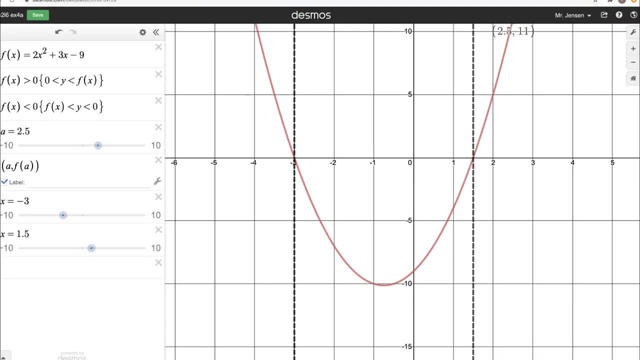 Okay, there's that function and I put vertical lines through the x-intercepts and notice when is the function positive? When is it greater than zero? In these two sections, when x is less than negative 3, and when x is greater than zero. So I can write that same answer in interval notation. by saying x is an element of numbers from negative infinity to negative 3, or from 1.5 to infinity. So I can write that same answer in interval notation by saying x is greater than zero when x is bigger than 1.5.. 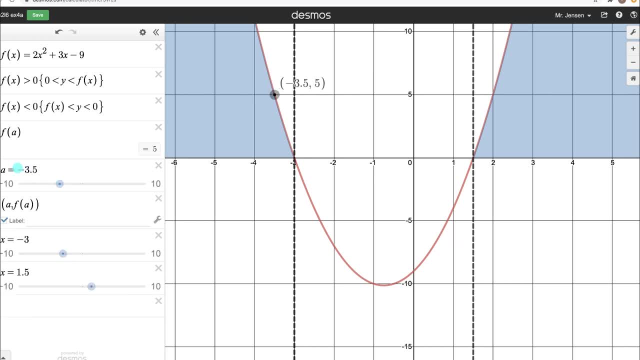 Also notice that when I have x-values in either of those two intervals I described, so either less than negative 3 or bigger than 1.5, look at the calculated y-value. You can see here, or on the point as well, The calculated y-values are all positive in that interval and in this interval. 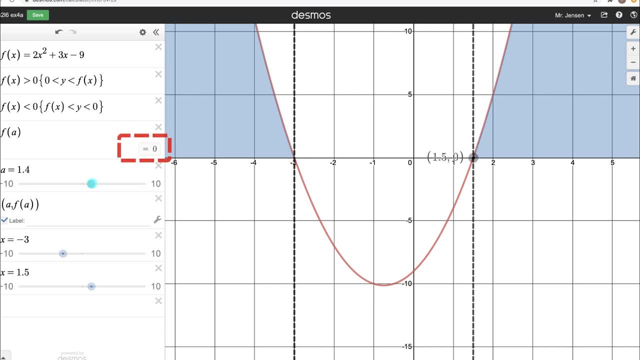 In the interval between negative 3 and 1.5, look at the calculated y-values: They're all negative And notice the x-intercepts are the positive, the place where the function changes signs. They don't necessarily always change signs at x. 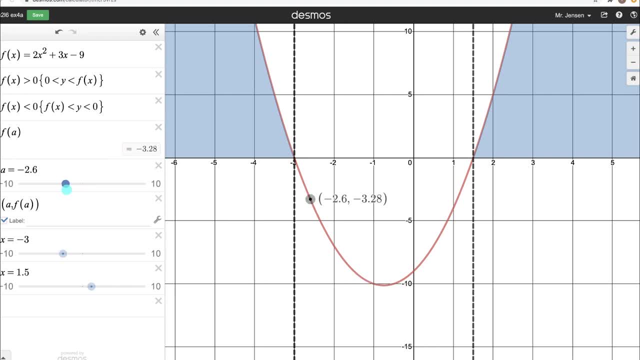 intercepts, but those are the places that it might change signs. So when we do method 2 to answer this question, where we make a factor table or sign chart, we are just going to pick test values for x in each of the intervals. So we'll pick a test value for x less than negative 3 for between. 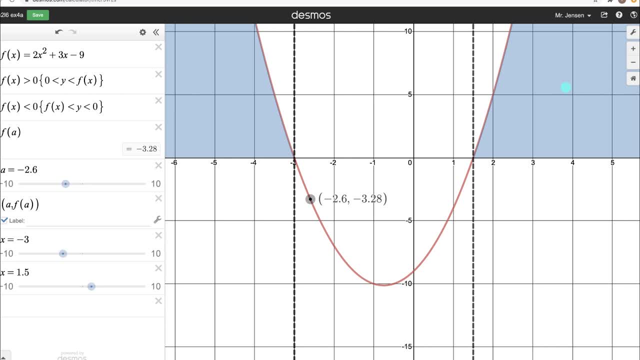 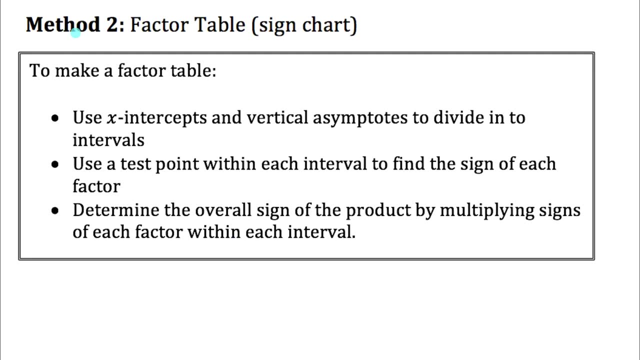 negative 3 and 1.5, and for bigger than 1.5, we'll plug in those test values into the equation and see what's the sign of the equation in each of the intervals. And that's what this describes here. Use the x intercepts, and this is, and vertical asymptotes. We don't have any of those. 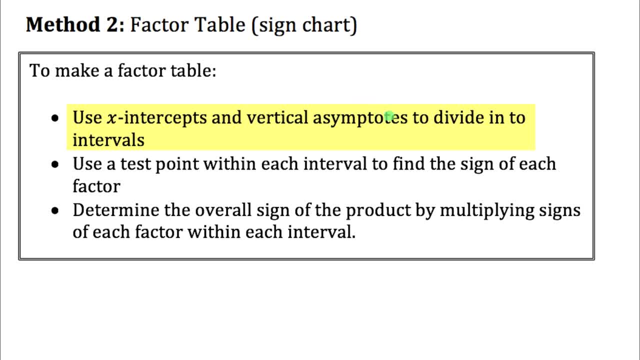 for polynomial functions. This is more. for once we get rational functions. later on in the course To divide into intervals, we'll pick a test point within each interval and we'll determine the overall sign of the function within each interval by plugging the x value into all of the factors. 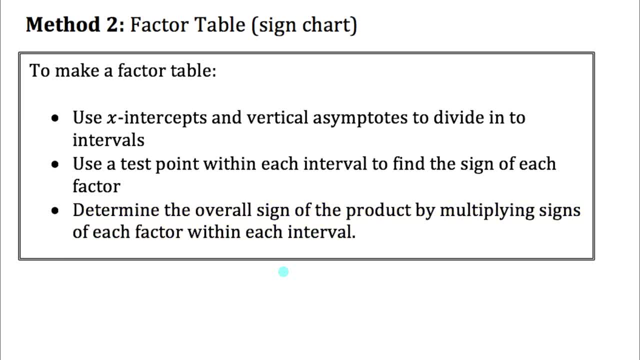 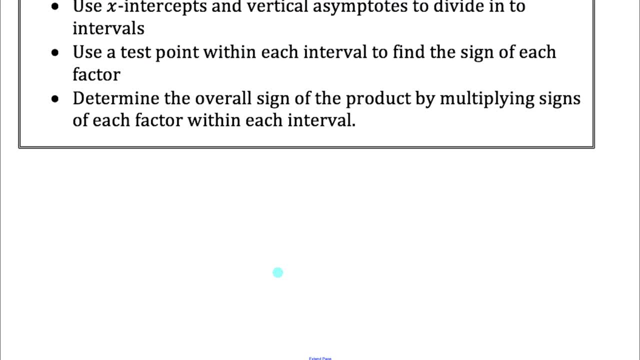 finding the product of the signs. I'll explain all that to you as we do our first example. So what are the x intercepts of the function? The x intercepts were negative, 3 and 1.5.. So when we make a factor table, we're going to need a vertical line for each of the x intercepts and 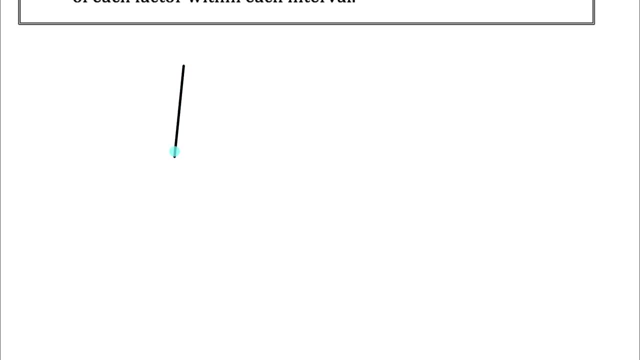 also one for negative infinity and positive infinity. So for this one we need four vertical lines— negative infinity, negative 3, 1.5, and infinity- And we are going to need a ROW for each interval. We still can measure whether or not an interval can be拉 trajectories. 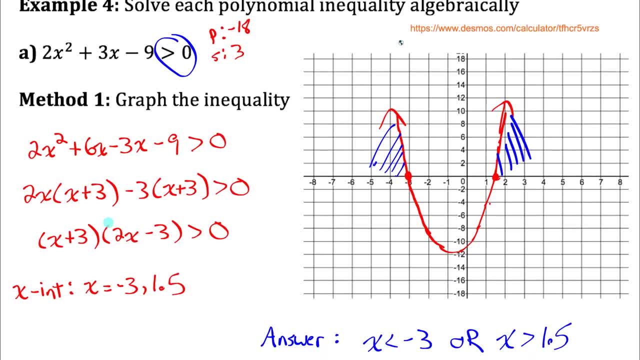 but this is a lived interception. We can see the function is wrong. the times, every Rhodes each of the factors of the factored form version of the equation. If we look at the factored form version of the equation, there are two factors, so I'm going to need two rows for this. 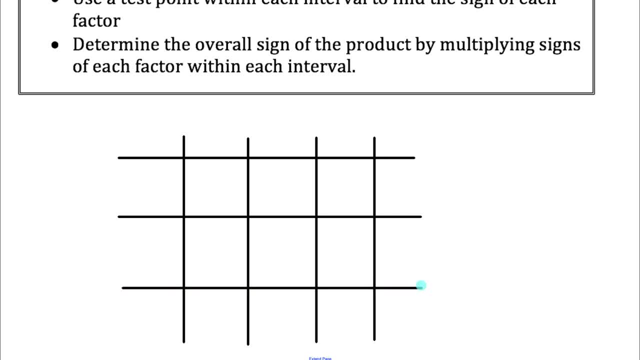 There's one row and here's my second row, So the table's a little bigger than I need it to be, but we can go with this. At the top of the table we are going to write the dividing points for each of the intervals. 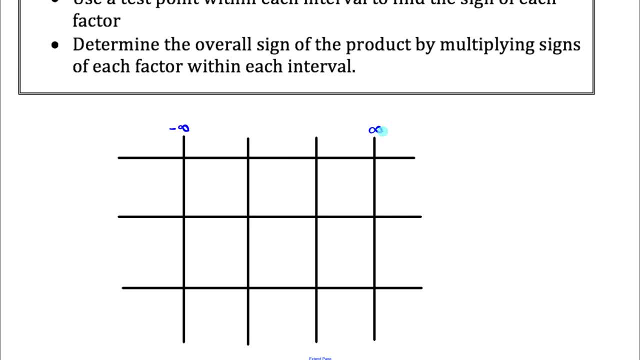 So always put negative infinity far left, positive infinity far right, and then the x-intercepts in between, making sure they're in ascending order. so negative 3 and 1.5.. And we write each of the factors here. So the factors were x plus 3 and 2x minus 3.. 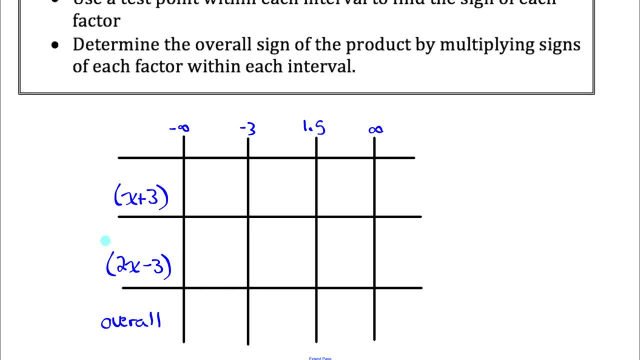 And I'm going to write the word overall here And now. we're just going to pick x values and plug them in. So let's pick an x value in this first interval. So the first interval is for x values between negative 8 and negative 3.. 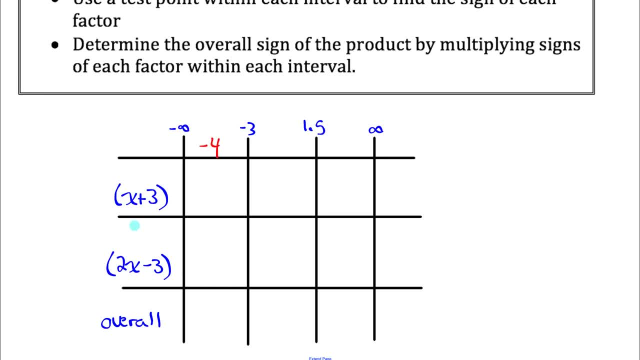 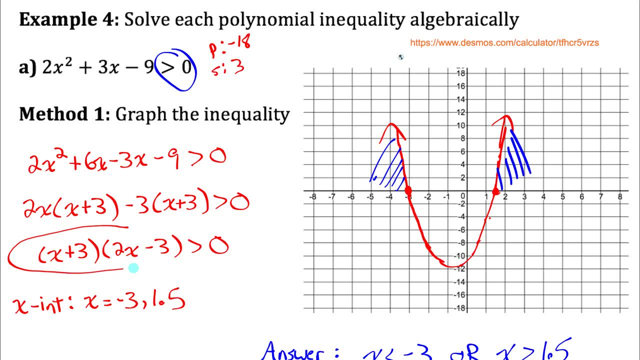 So let's pick any x value in that interval. I'll pick negative 4.. That negative 4 is our test value. We're going to plug that in to this function, which is just the factored form version of that, And we're going to use that to figure out what's the sign. 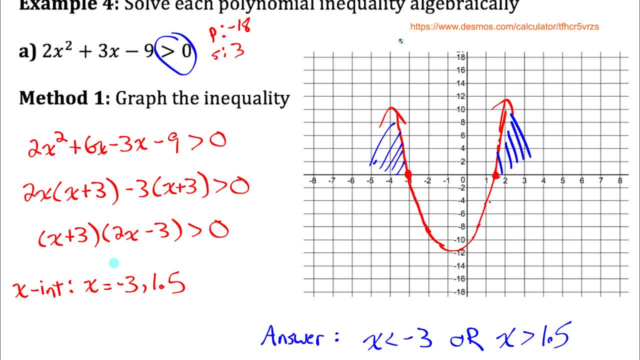 Now I don't care the actual value, I just want to know: is it positive or negative? And I can figure that out by figuring out. well, does it make the first factor positive or negative? Does it make the second factor positive or negative? 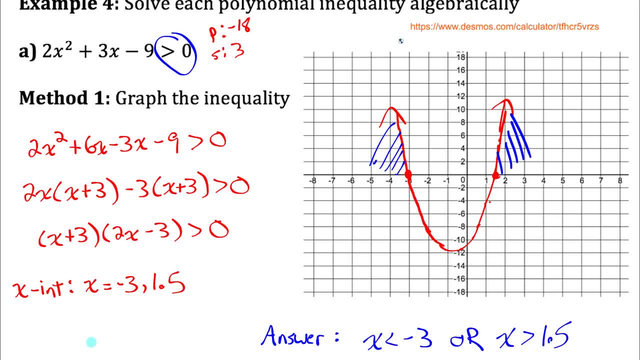 And then I can just multiply those signs together and figure out. well, is the overall value positive or negative? So what does it do to x plus 3?? Once I plug negative 4 into x plus 3, I would get negative 1.. 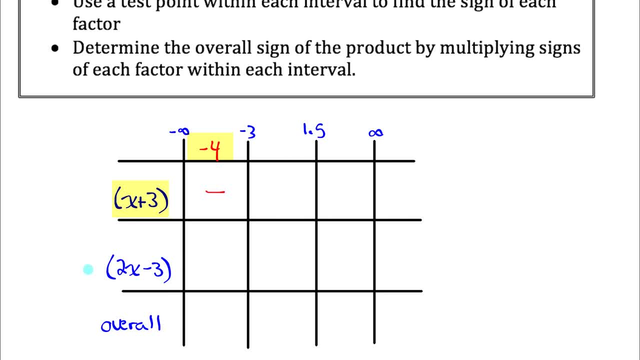 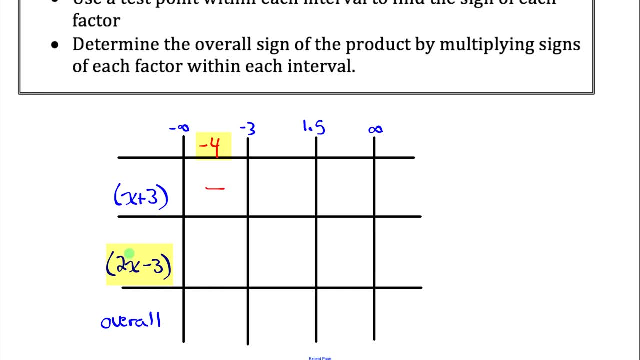 I don't need to write negative 1.. I don't care the actual value, I just care that it makes that factor negative. What does it do to the second factor? What does it do to 2x minus 3?? If I plug negative 4 into 2x minus 3, I would get negative 11.. 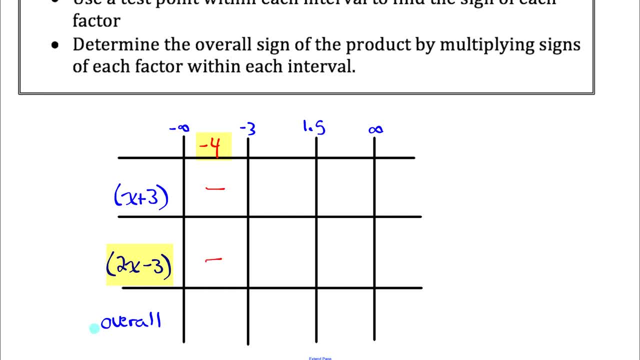 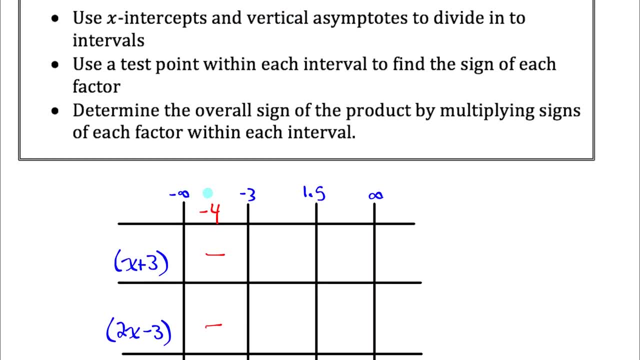 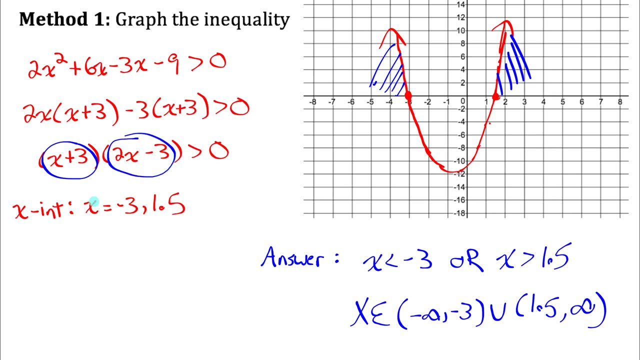 Once again, I don't care that it's negative 11.. I just care that it's negative. So what this tells me? when I plug negative 4 or any x value in that interval from negative infinity to negative 3, it will make this factor be negative and this factor be negative. 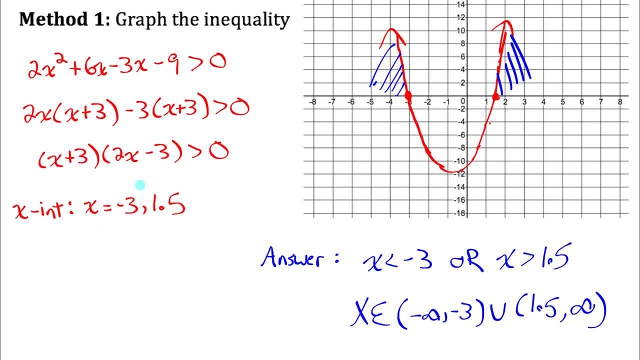 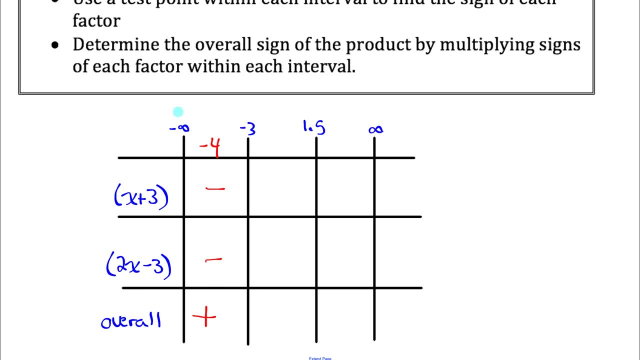 So I would have a negative times, a negative. That's positive. An even number of negative factors is going to give you a positive result. So I figured out within the interval negative infinity to negative 3, the function is positive. It's above the x-axis. 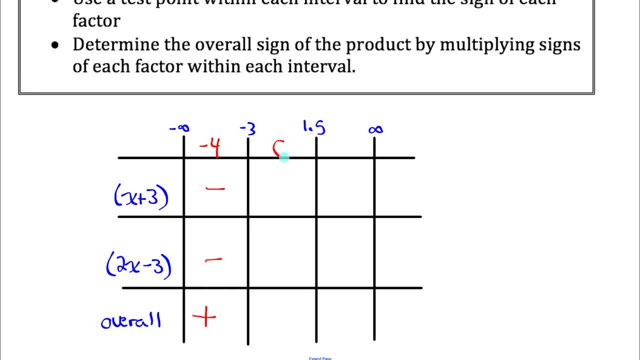 How about between negative 3 and 1.5?? Let's pick a test value. How about 0? 0. 0. 0. 0.. I would plug 0 into both of those factors. Into the first factor, I would get 3,, which is positive. 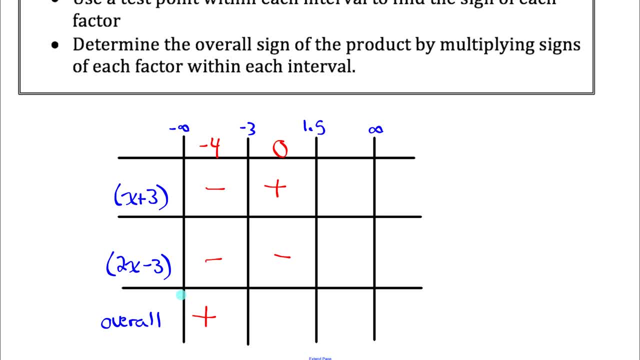 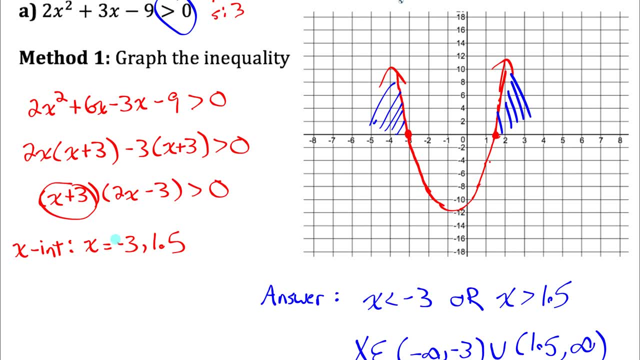 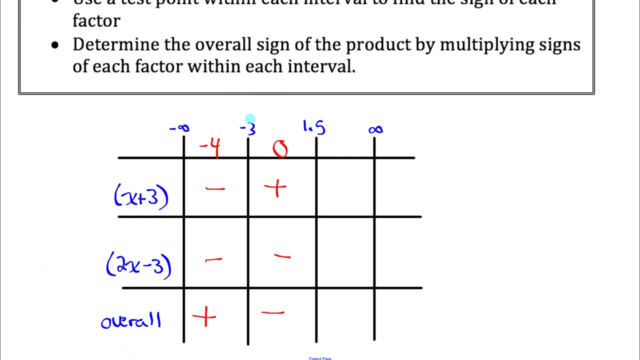 Into the second factor, I would get negative 3, which is negative. So that means in the equation I would get a positive times a negative And a positive times a negative is negative. So that means within the interval of x values, from negative 3 to 1.5,. 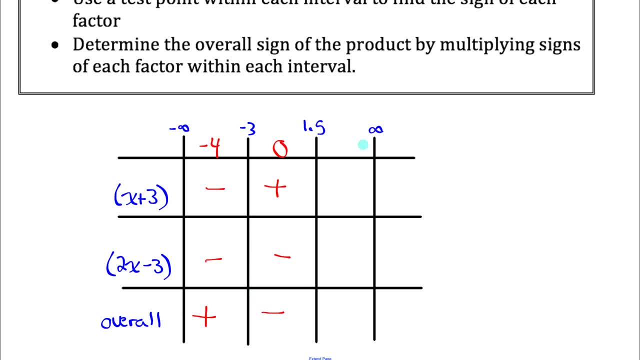 the function is negative. How about from 1.5 to infinity? Pick any number. Pick any number in that interval you want, I'll pick 2.. Plug it into both factors. Into the first factor, I would get 5,, which is positive. 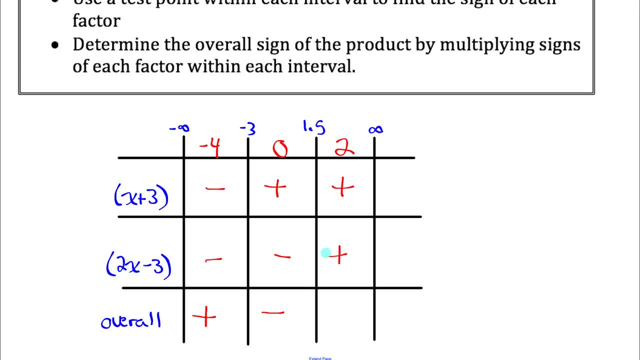 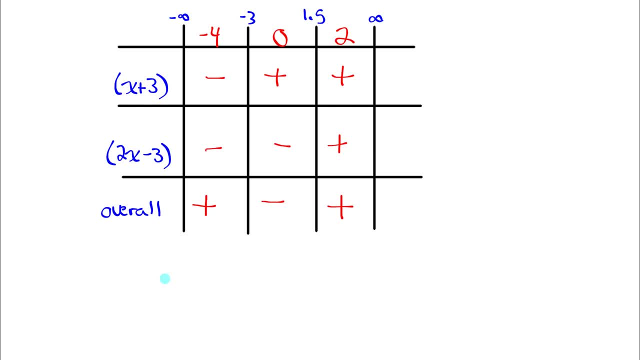 Into the second factor, I would get 1, which is positive. So a positive times a positive is positive. So if you look at this factor table, it actually shows us our answers Because, remember, the original question wants to know when is the function greater than 0?. 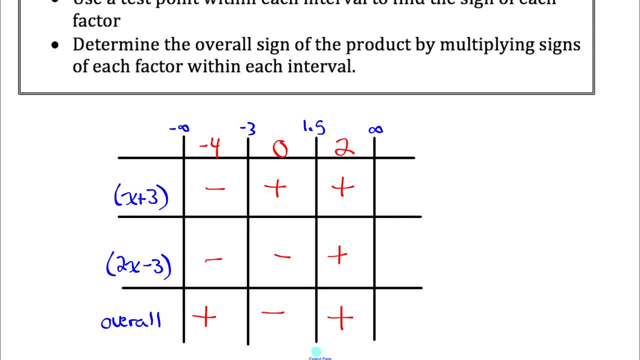 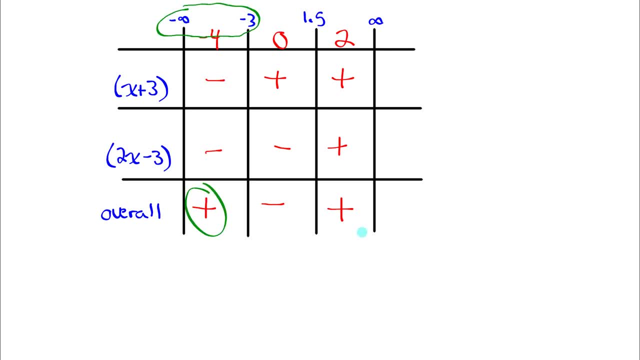 Which means when is it positive? And if we look, the function is positive in this interval from negative infinity to negative 3.. And it's positive in this interval from 1.5 to infinity. And look at how we wrote our answers. 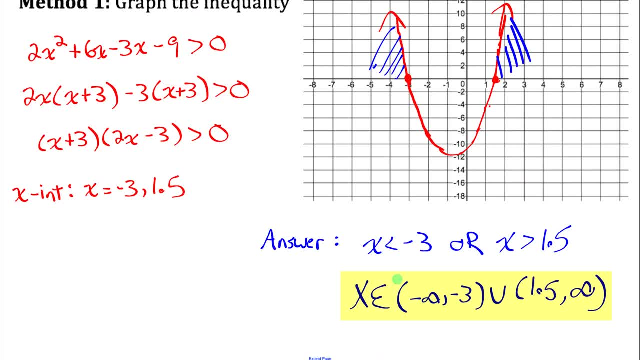 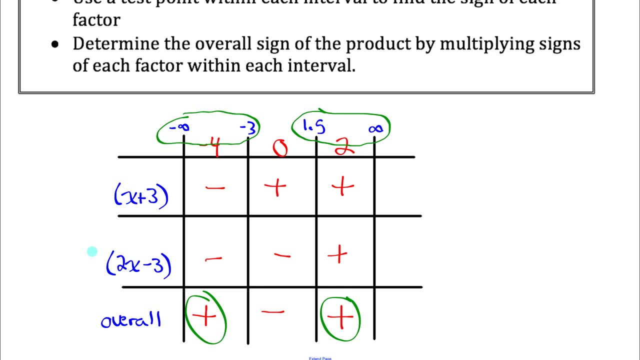 Our answers are literally those two intervals written Negative infinity to negative 3, or 1.5 to infinity. So do you see how the factor table shows us our answers? Let's do another example where we'll solve it both ways: graphically and with a factor table. 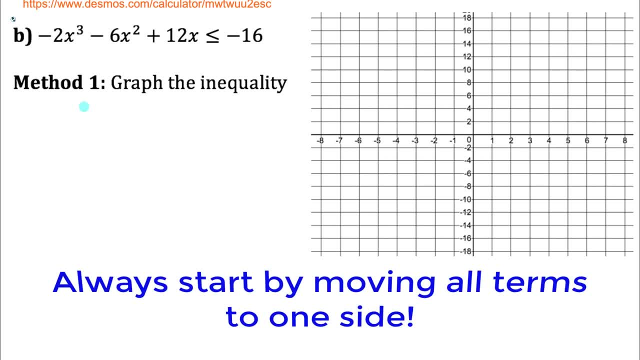 Step one for these polynomial inequalities is always: move everything to one side. So we'll move all the terms to the left for this one. So let's add 16 to both sides. So I've got negative 2x cubed minus 6x squared, plus 12x, plus 16 less than or equal to 0.. 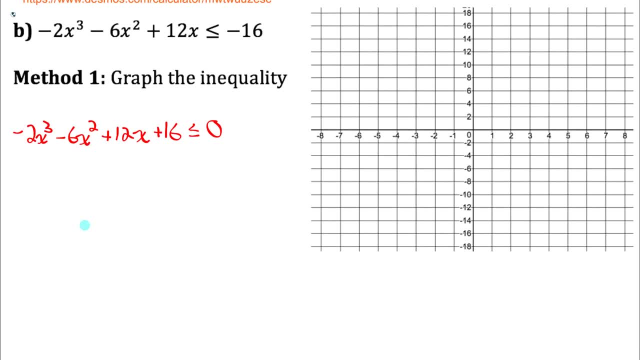 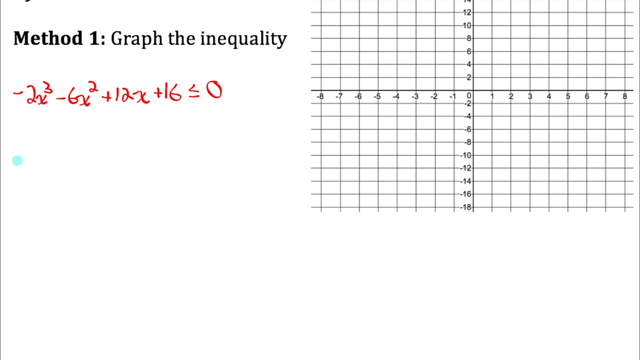 Okay, the first thing we should always do whenever we're trying to factor something is check for common factors. I'm going to take a negative 2 out from all terms. All of the coefficients are even numbers, so I can take out a 2.. 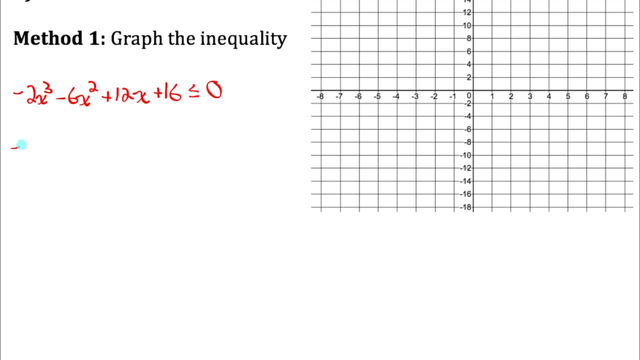 I'm going to take out a negative 2, since the leading coefficient is negative, So negative 2, and then divide each term by negative 2.. I have x cubed plus 3x squared minus 6x minus 8 is less than or equal to 0.. 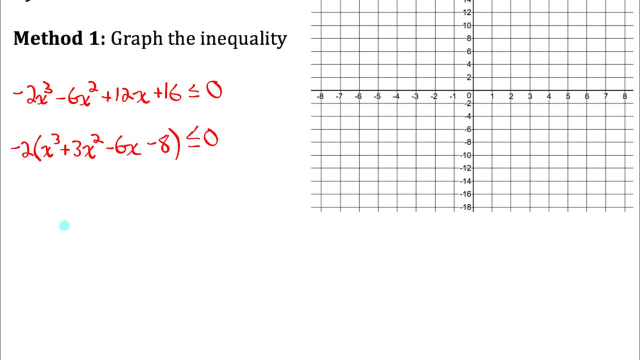 Now I could divide both sides of this by negative 2 to get rid of this negative 2, but then I'd have to reverse the inequality sign. So, to keep this as uncomplicated as possible, I'm not going to do that. 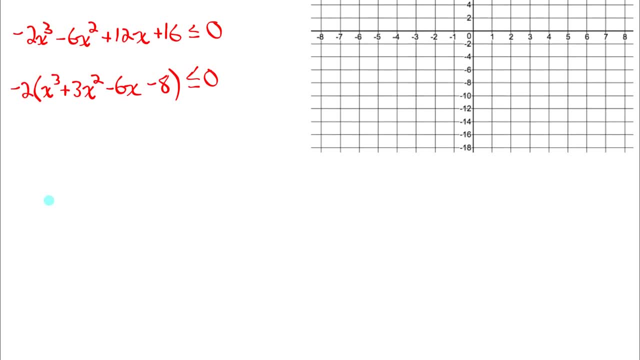 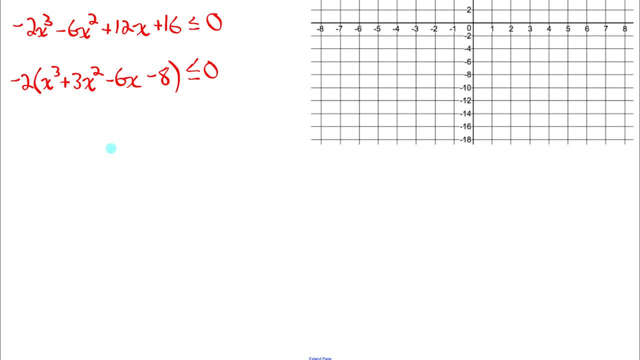 I'm going to leave that negative 2 there And now what I'm going to do is focus on this factor in brackets and see how can I factor this. Well, it's four terms. You could try factoring by grouping. In this case it's not going to work. 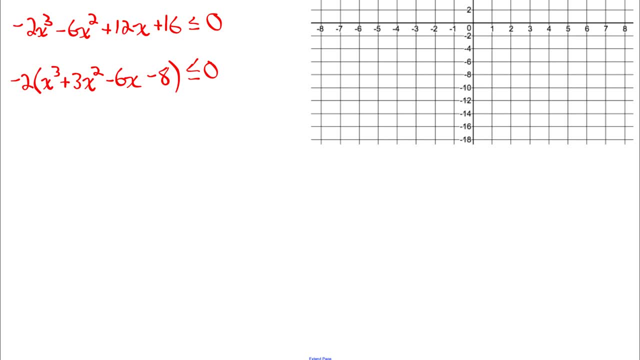 So we'll have to use our factor theorem and test for zeros and do synthetic division. I'm going to call this function in brackets, function f at x, just to make it easy, And we're going to try and figure out what could make that be zero. 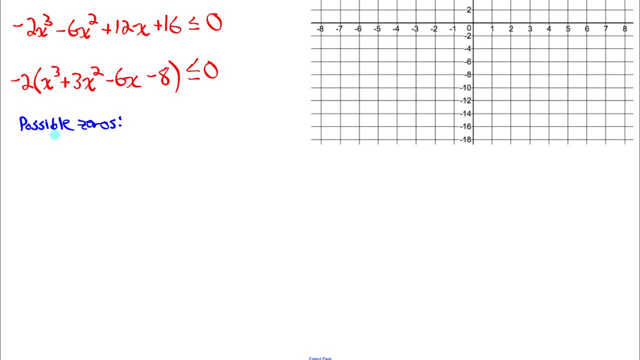 So I'll write possible zeros Based on the integral zero theorem. I know an integer that would make this be zero would have to be a factor of the constant term. So factors of eight are plus or minus one, two, four or eight. 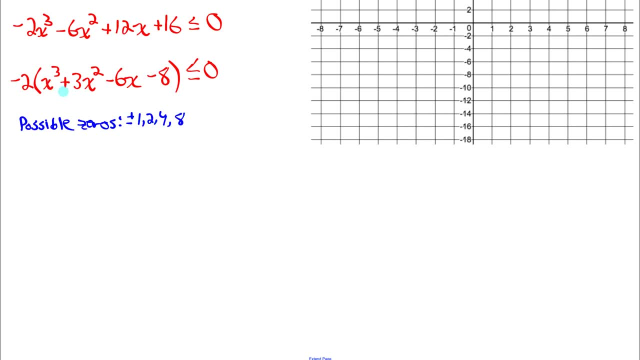 And I just need to find one number that makes this be zero. One doesn't work, Negative one. If I plugged in negative one, negative one cubed is negative one plus three times negative one squared. So plus three minus six times negative one. 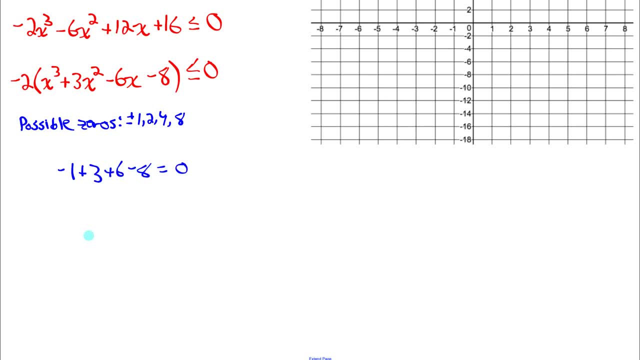 That's plus six, Minus eight, eight, that's zero. So I just did a little test there and I figured out that negative one makes it be zero. So I'm going to say f at negative one equals zero. That tells me that x plus one is a factor. 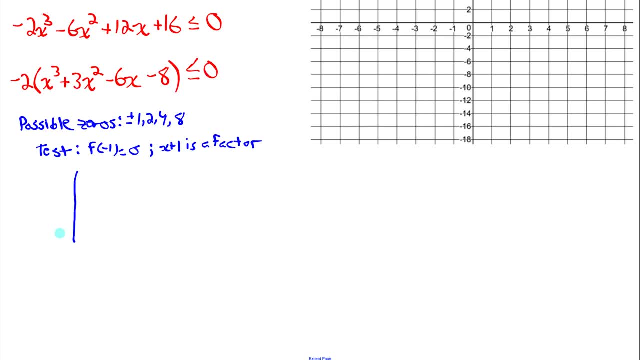 So what I can do is divide that polynomial by x plus one. So I'll just set myself up a little synthetic division table, put negative one here, because that's the zero of the divisor, And write the coefficients of the polynomial across the top. 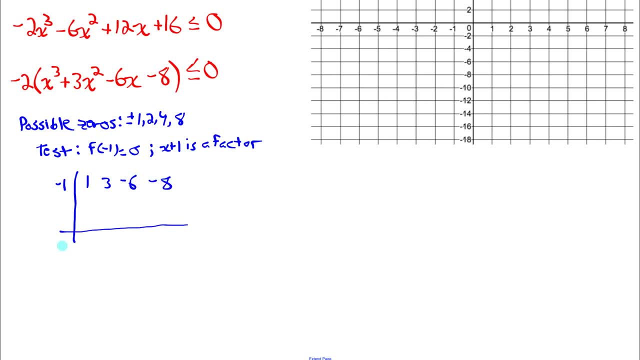 So one, three negative, six negative, eight. And then do my synthetic division. quickly Bring down the one: multiply by negative one, add get two. multiply by negative one, add, get negative eight. multiply by negative one, add, get zero. 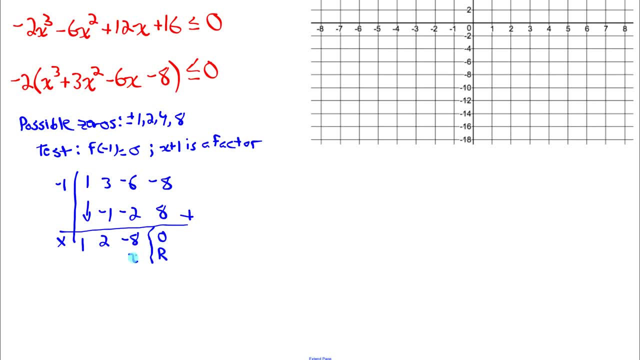 So I've got my remainder and the coefficients of my quotient are here: Coefficient of x to the zero, of x to the one and of x squared. So now I can go back to what I was doing here and rewrite this x cubed factor in factored form. 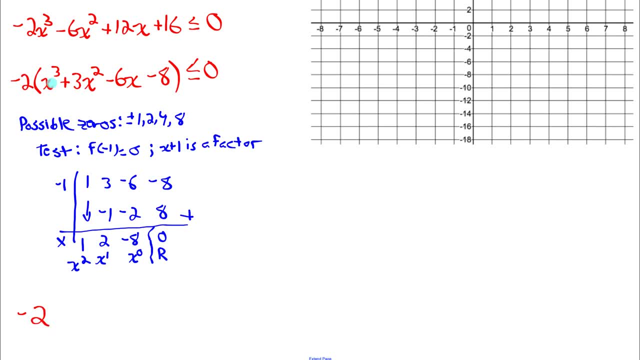 So this negative two is still here. Don't forget about the negative two. But I can rewrite this x cubed function as a product of the divisor x plus one and its quotient x squared plus two x minus eight. And I'm interested in when is this less than or equal to zero? 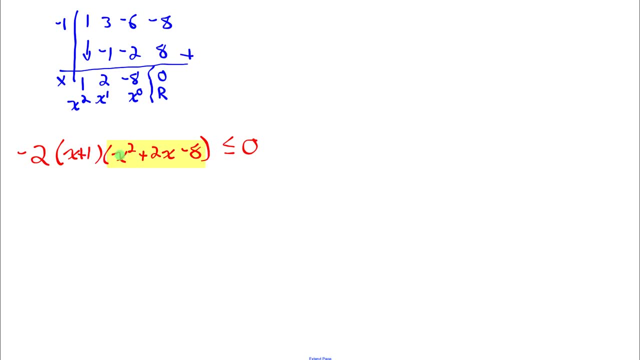 This x squared plus two, x minus eight is a quadratic, So this factor is higher than degree one. So we should try and factor it further. Are there numbers that multiply to negative eight and add to two? Yes, those numbers are four and negative two. 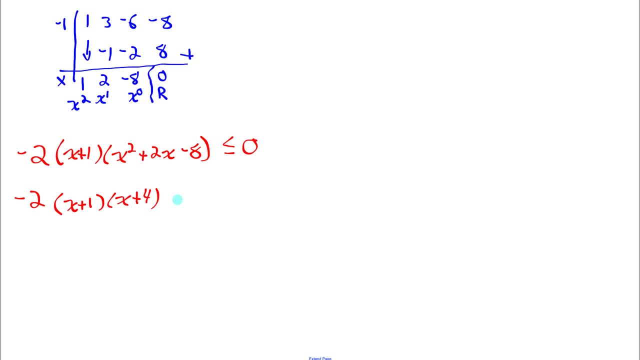 So it would factor to x plus four times x minus two. OK, that's now fully factored form. All the factors are degree one, so I know I can't factor further From that factored form version of the inequality. I can now state what the x intercepts would be. 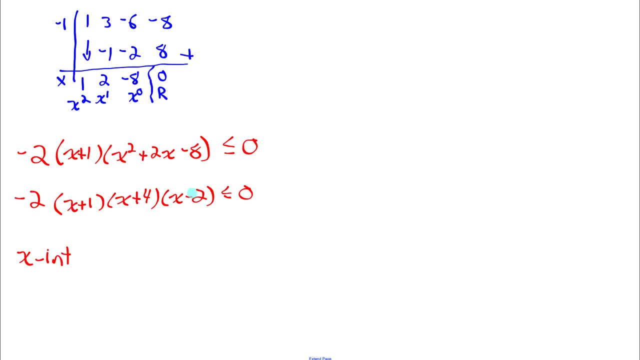 What x values would make the left side of this inequality be zero. From the x plus one factor, I know negative one would make the product be zero. From the x plus four factor, I know negative four would make the product be zero. And from the x minus two factor, I know two would make the product be zero. 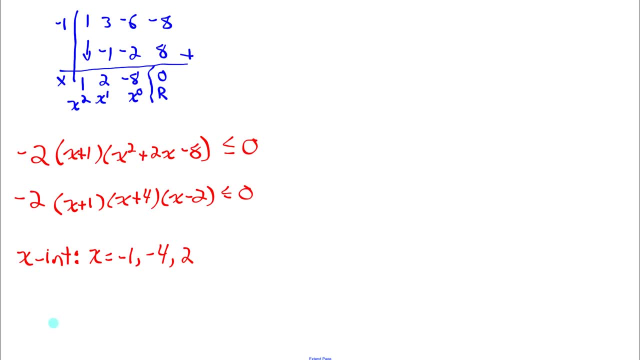 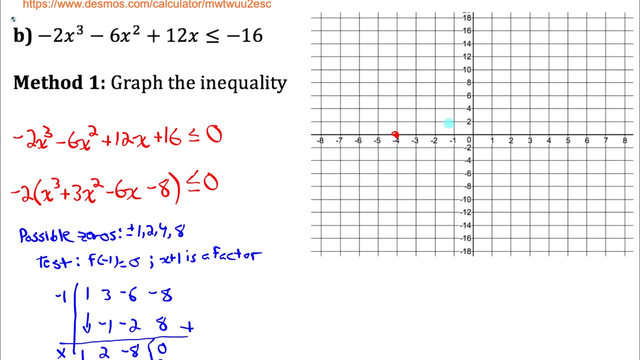 So those are the x intercepts. So with that information we now have two options. We can solve this graphically or using a factor table. Graphically, we would plot the x intercepts. They were negative, four negative one and two. 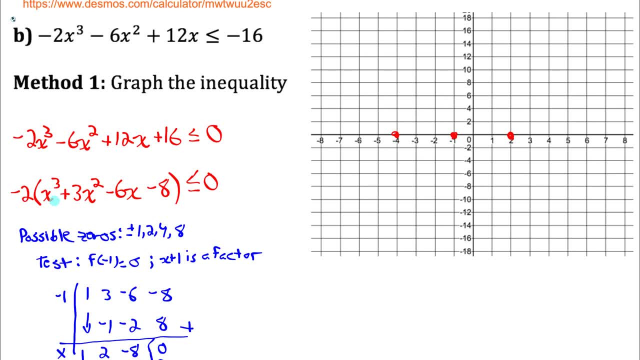 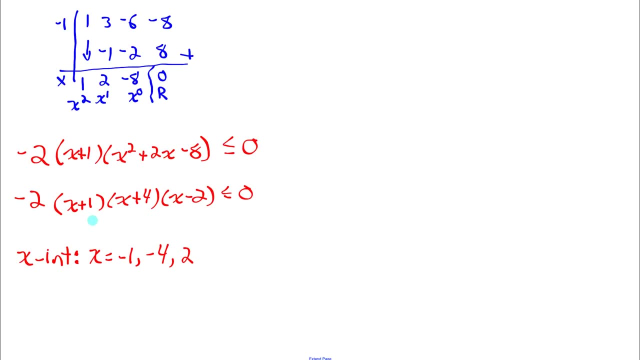 And then we would do a rough sketch of the function based on its end behavior. Well notice, this is odd degree negative leading coefficient. Odd degree negative leading coefficient. I know it's going to go from quadrant two to quadrant four And each of the x intercepts. if we look at the factored form version. 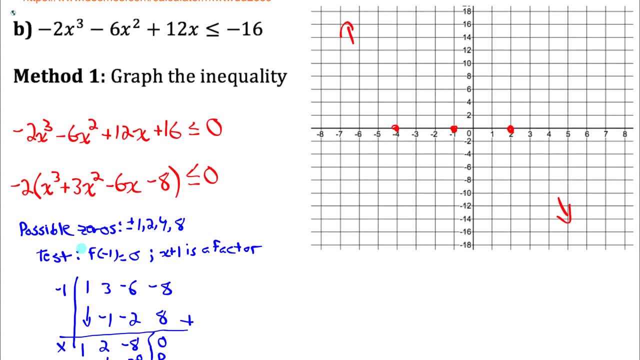 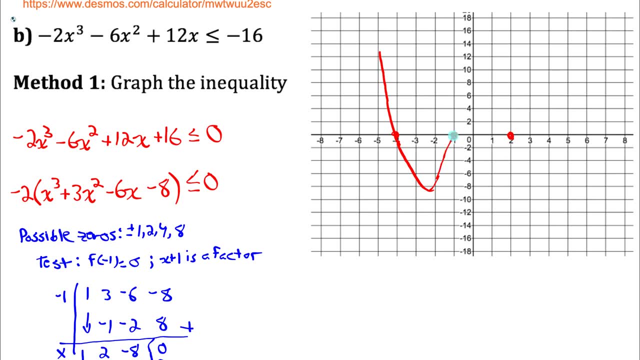 we're all order one. So I know it's going to go straight through each of those x intercepts. So it's going to go something like this, And I know this isn't perfectly accurate, but that's OK. So once we get the correct intervals, 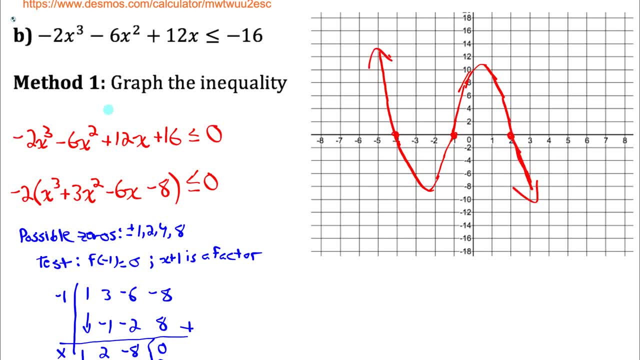 of where it's positive and negative. that's all we care about. There's a rough sketch of the function that has the correct x intercepts and end behavior. We should now be able to answer the question We're interested in: when is the original? 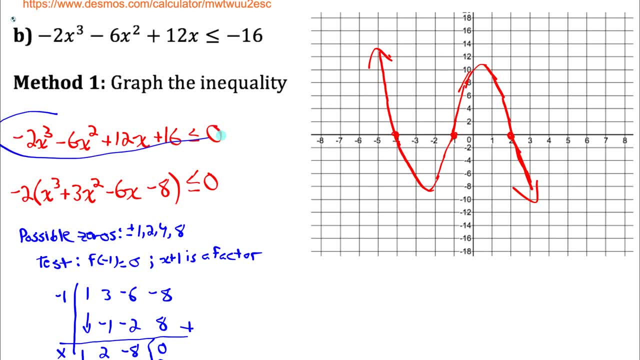 function less than or equal to negative 16, but we rearranged it to get this, So the answers to that inequality are going to be the same as the answers to the original one. So, really, what we're trying to do is answer this once it's all rearranged to one side. 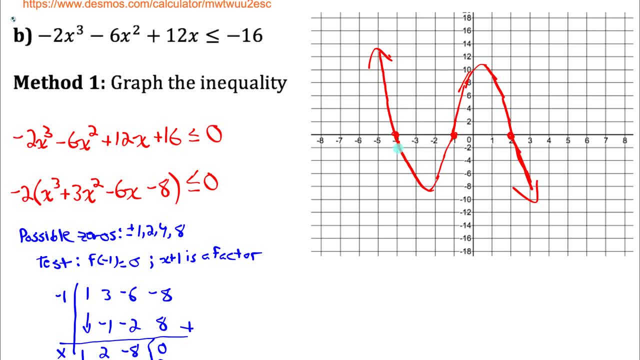 So when is it less than or equal to zero? So when is this function negative? It's negative here and here. So we just have to describe those two intervals, So between negative four and negative one, and also greater than two, And notice the equal sign under the inequality. 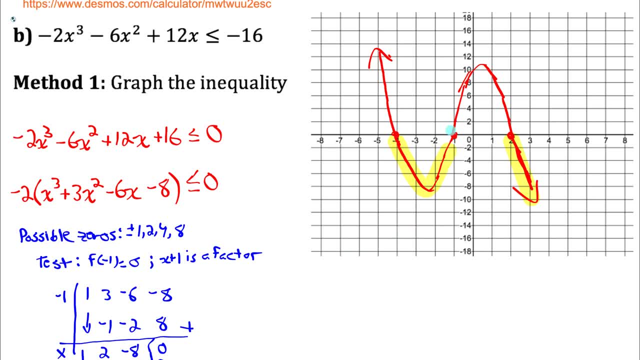 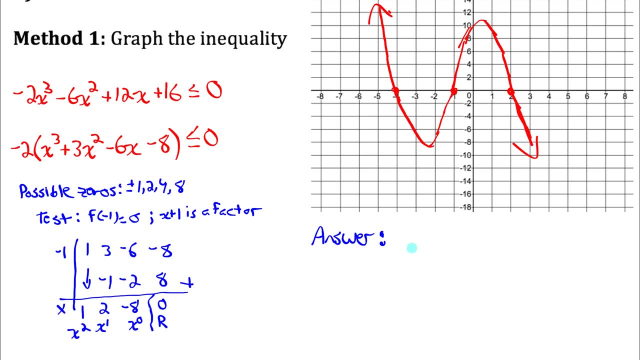 So we want to include when is it equal to zero as well. So we have to include negative four, negative one and two in our answers. Answer: the original inequality is true when we have an x value between negative four and negative one, including those two. 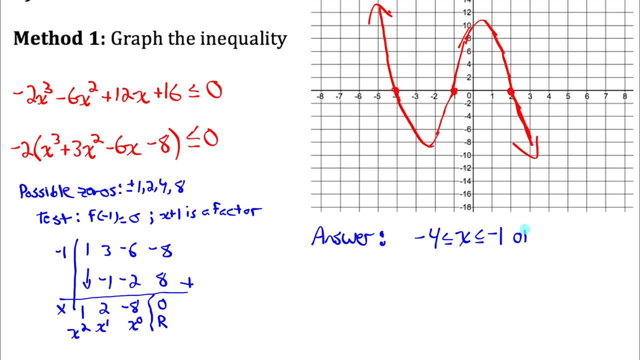 x values Or an x value greater than or equal to two. In interval notation we'd say x is an element of numbers between negative four and negative one, or from two to infinity. And notice the square brackets at each of the x intercepts, because those x 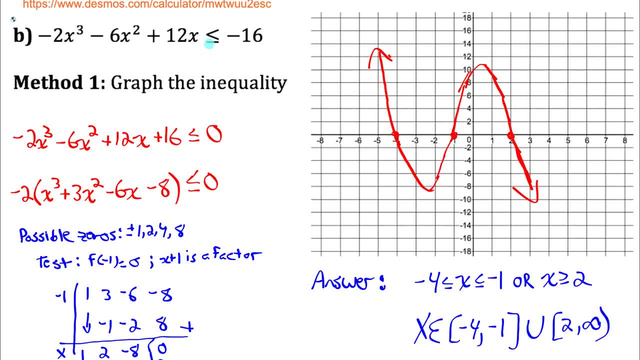 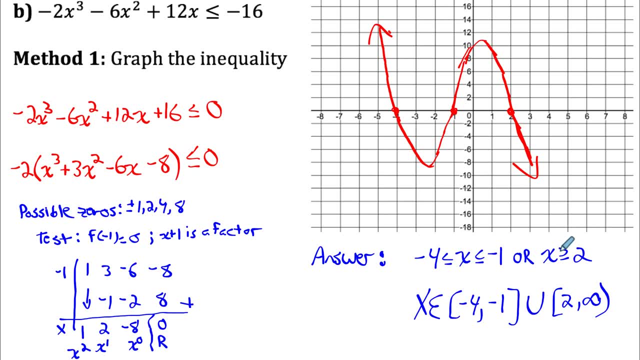 intercepts make it be zero and we want to include: when is it equal to zero? because of that equal sign under there. And just to make sure you really get what's happening here, like, for example, this interval: x greater than or equal to two, if we picked an x value greater than, 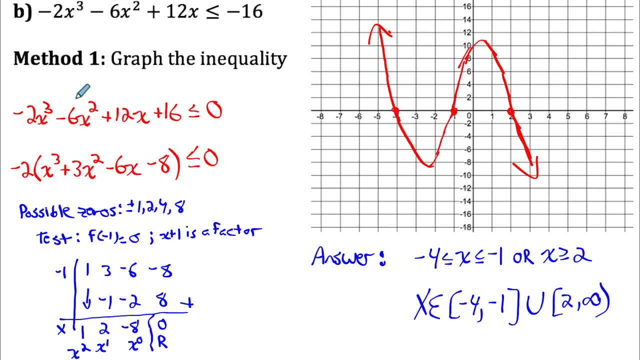 or equal to two, so let's say three, it would make this inequality true. We'd get an answer that was less than or equal to zero, which means it would make this inequality true, which means the left side would be less than, or equal to negative, 16.. But it's way easier to solve when something 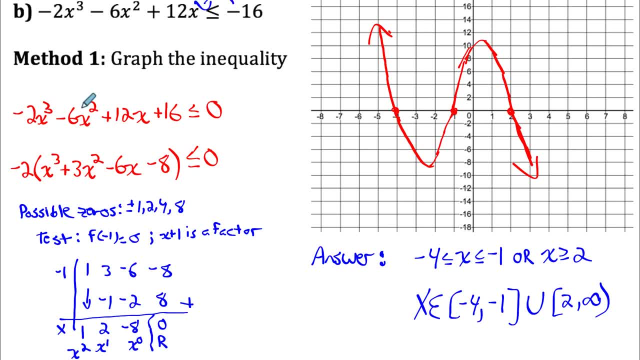 is less than or equal to zero. That's why we do the rearranging, So we're going to do the first and then solve this inequality. The solutions to that inequality will be the same as the solutions to that inequality. Let's look at how we could have got this answer algebraically. 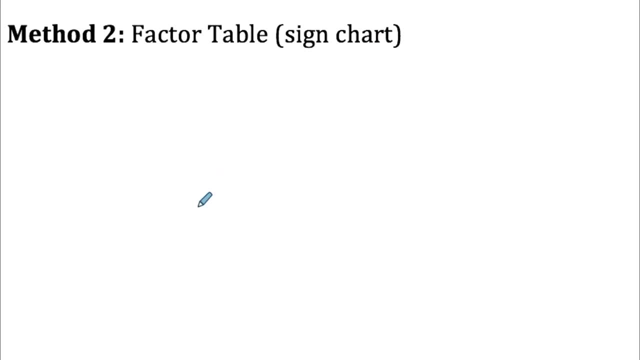 So we can make our factor table or sign chart and then test values within each interval. So, because there are three x intercepts, this time I'm going to need to draw five vertical lines- negative infinity- each of the three x intercepts. 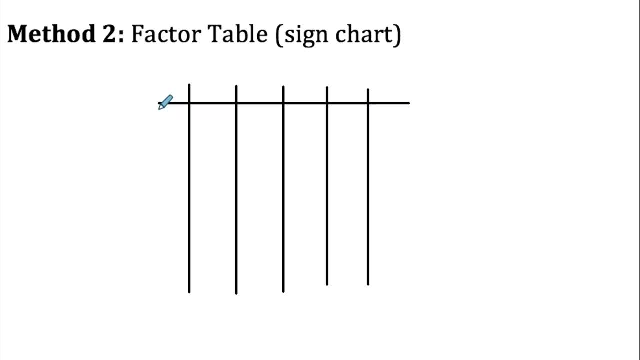 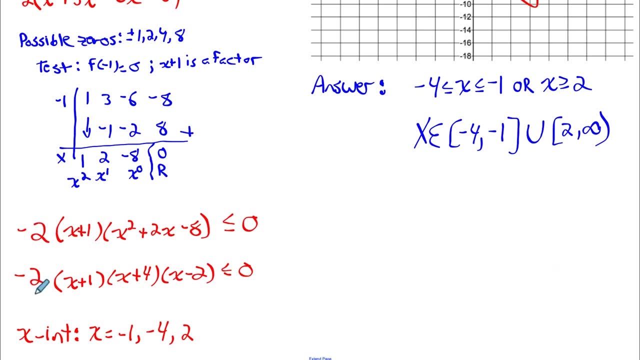 and then positive infinity. And then I need a row for each of my factors in my factored form version of the equation And notice the factored form version. There are one, two, three, four factors. Don't forget about that factor of negative two. 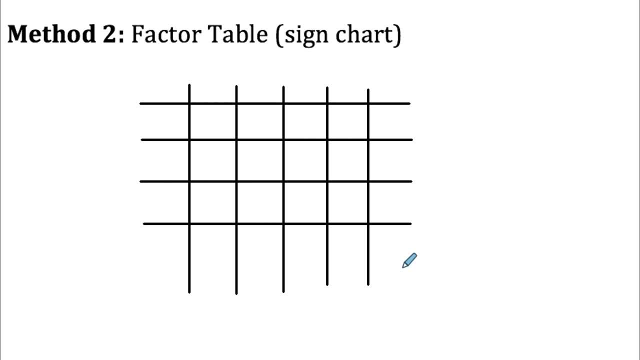 So I'm going to need to know four rows, One So negative. infinity to infinity Always go far left and far right And then between need to be the x intercepts in ascending order. So I believe they were negative four. negative one. 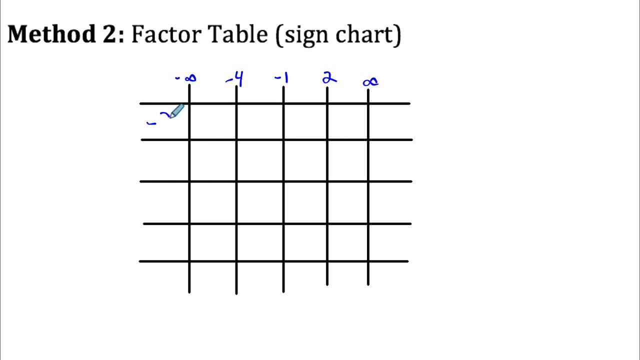 Negative two, And on the left side we need all of the factors, not forgetting to put that factor of negative two. So negative two, X plus four, X plus one And X minus two, And I don't know why I'm keeping the brackets there. 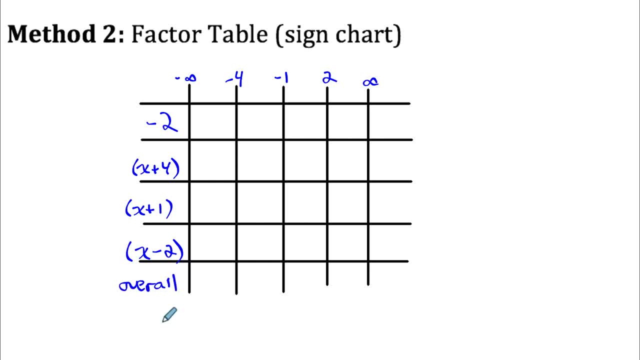 You don't need them And I'm going to put overall down here where we comment on the overall sign of the entire function And now we just test values. Let me just move over to Desmos to show you what we're doing here. 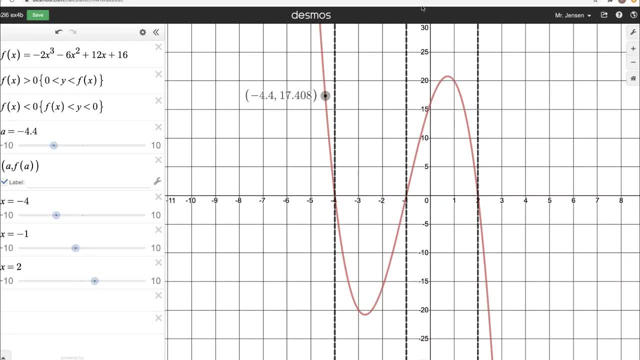 So here's the function. I've got vertical lines through each of the x intercepts. Those are the dividing points of the intervals, And then we're just picking an x value within each interval and testing what's the sign of the function in that interval. 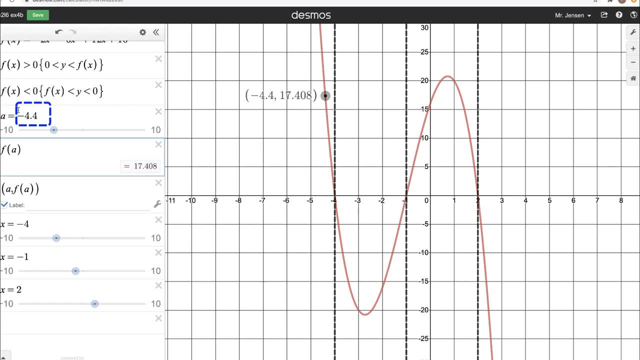 So I've got my x value here right now It's negative four point four. plugged into the equation It calculates seventeen point four zero eight. So it gives me that point right there. Notice that point is above the x axis has a positive y value. 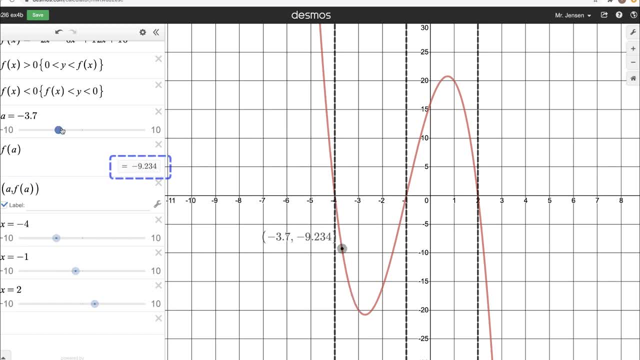 In the next interval between negative four and negative one, any x values in that interval will give us a negative y value. And then, from negative one to two, all the y values are positive, And then from two to infinity, all the y values are negative. 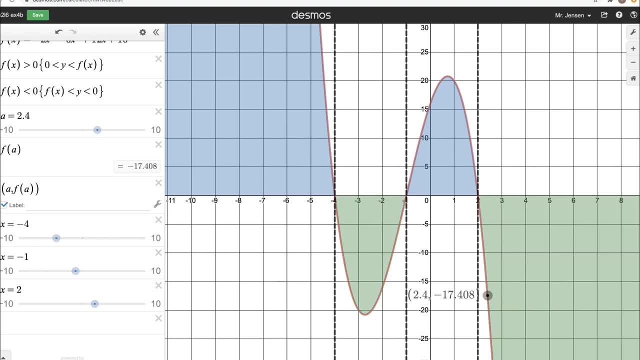 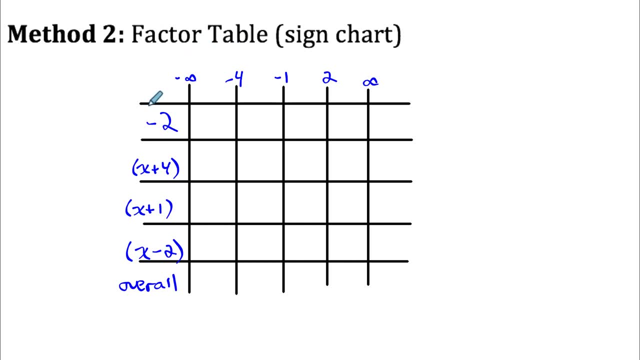 So you can see the intervals from where the function is positive and where the function is negative. We're just testing that out algebraically. So let's pick an x value in that interval between negative infinity and negative four, And any x value works. 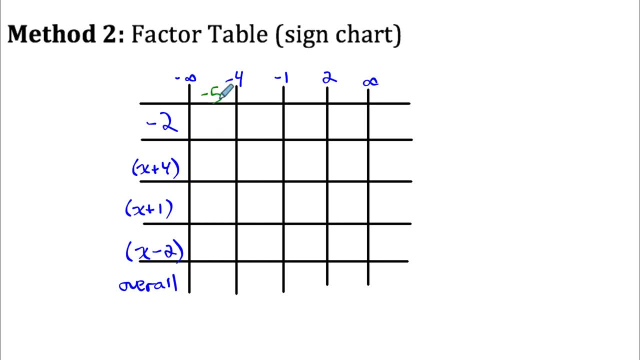 How about negative five? That negative five plugged into each of the factors. what sign does it make each of the factors? Well, negative two is always negative. I could just fill out that entire row right now. That's not going to change. based on an x value. 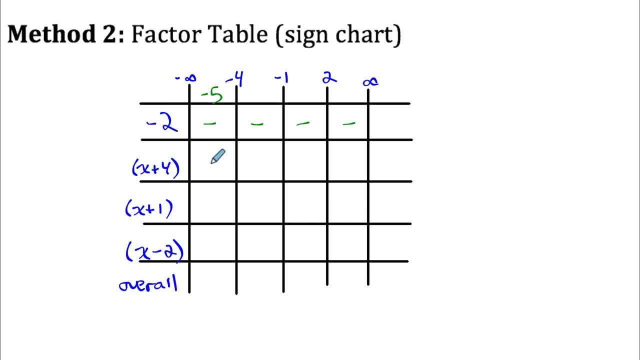 There's no x with it, But when negative five goes into x plus four, I get negative one. When negative five goes into x plus one, I get negative four. And when negative five goes into x minus two, I get negative seven. 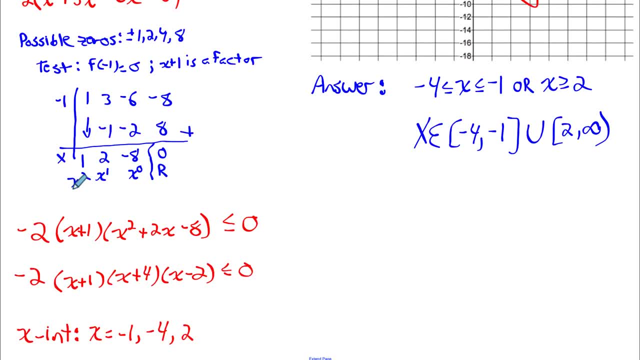 So what does that do to the entire left side of the inequality? I would get a negative times a negative times a negative times a negative. I don't care what the values of those are, I just care that they're all negative And the product of four negative factors is positive. 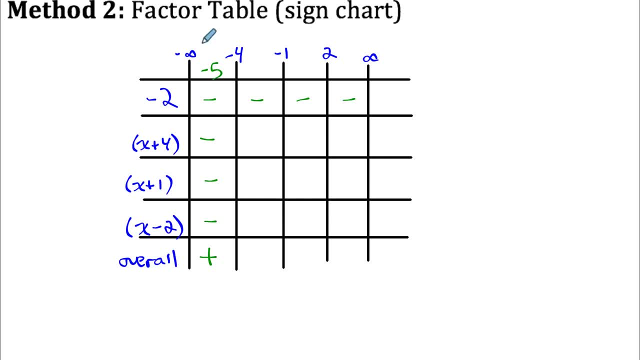 An even number of negative factors gives us a positive result. So the function is positive in the interval from negative infinity to negative four. How about negative four to negative one? Let me pick an x value in that interval, So negative two. What does it do to each of the factors? 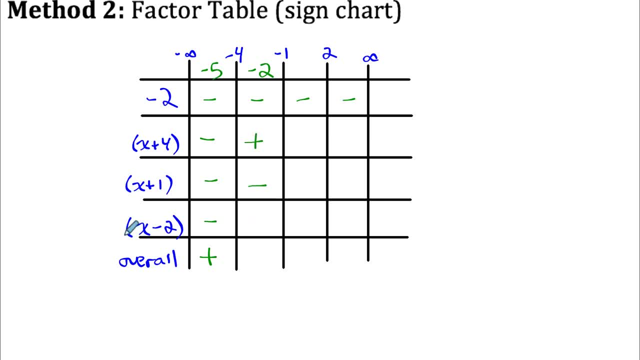 Well, it makes x plus four be positive, It makes x plus one be negative and it makes x minus two be negative. I have an odd number of negative factors which gives me a negative result. The next interval from negative one to two, I'll pick an x value of zero. 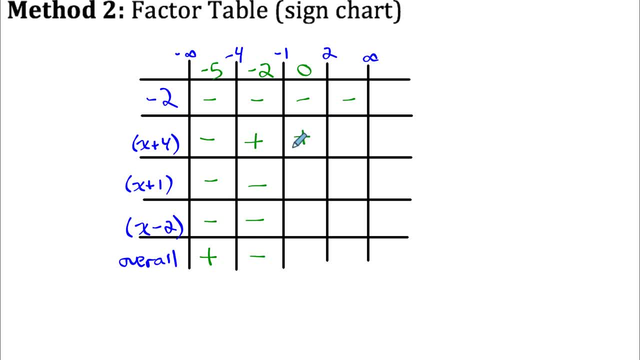 Plug it into all of the factors: Zero plus four is four, Zero plus one is one and zero minus two is negative. two Even number of negative factors is a positive result And the last interval from two to infinity, I'll pick an x value of three. 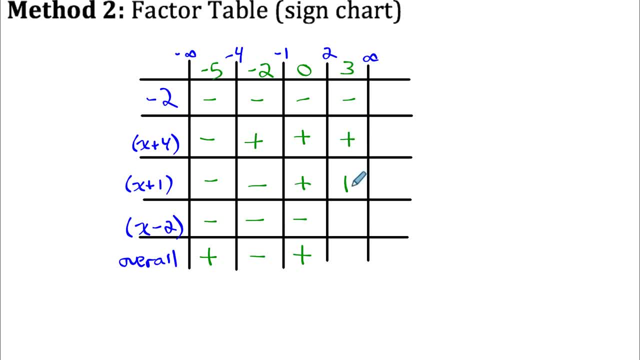 Three plus four is seven, Three plus one is four and three minus two is one. An odd number of negative factors, right? There's just one negative factor, negative result, And we want to know when is that function less than or equal to zero? 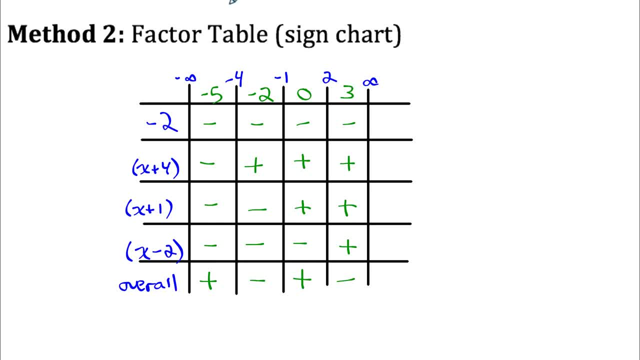 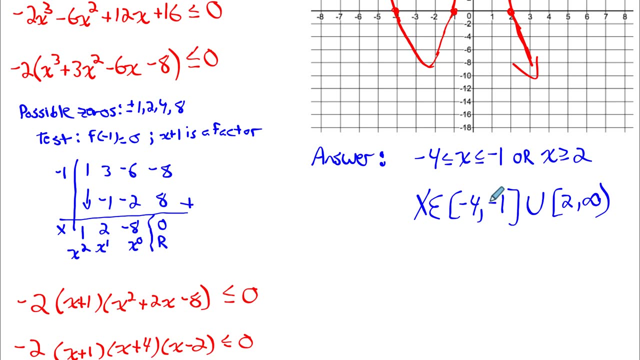 Which means when is it zero or negative? Well, it's negative in this interval and this interval. And if you look at our answers, we wrote from negative four to negative one and from two to infinity. Here they are: Negative four to negative one, two to infinity. 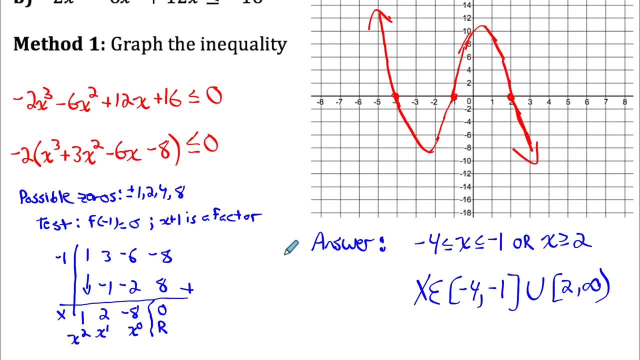 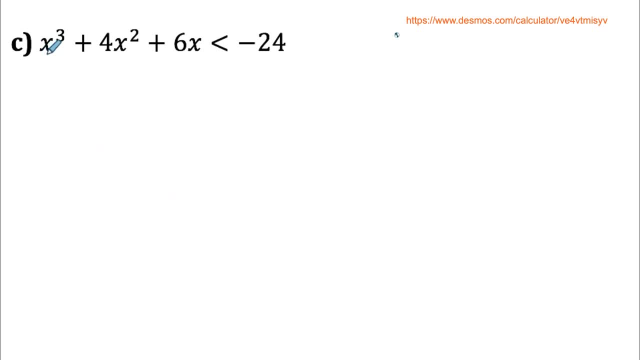 And we included all of those x steps with square brackets because of the equal sign underneath the original inequality symbol. Here's our last one. Let's start by doing step one and rearranging this so all terms are on one side. So to answer this inequality, we could rearrange it. 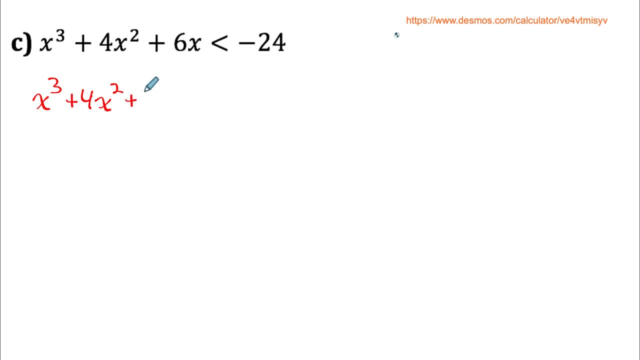 to x cubed plus four, x squared plus six, x plus twenty four, less than zero. So whenever this is less than zero, that's when this will be less than negative four. So how can we figure out when this is less than zero? Well, we need to get it into factored form. 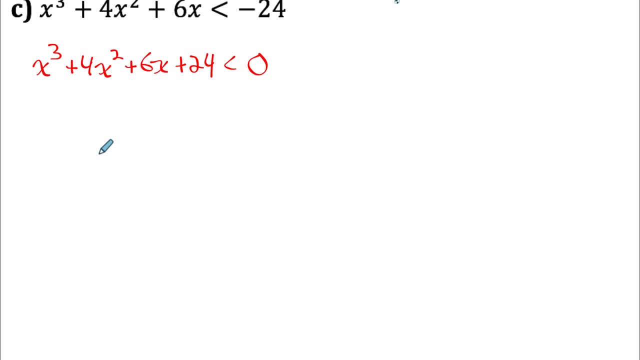 And hey, there's four terms here. I should try factoring by grouping. It might make this one easier, And in fact I think factoring by grouping works. If I common factor from the first two terms in x squared, I would get x plus four. 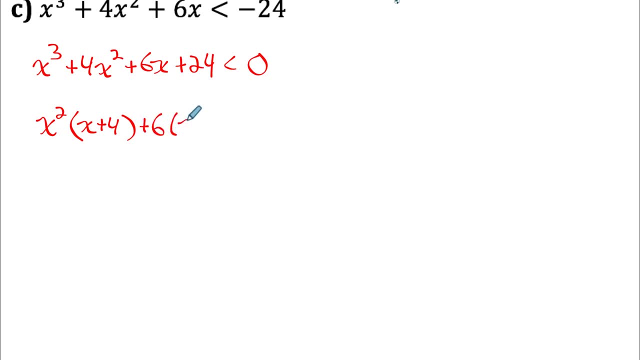 And from the last two terms. if I took out a six I would get x plus four. It's a common binomial which means I can common factor out that common binomial And be left with x squared plus six is my second factor. 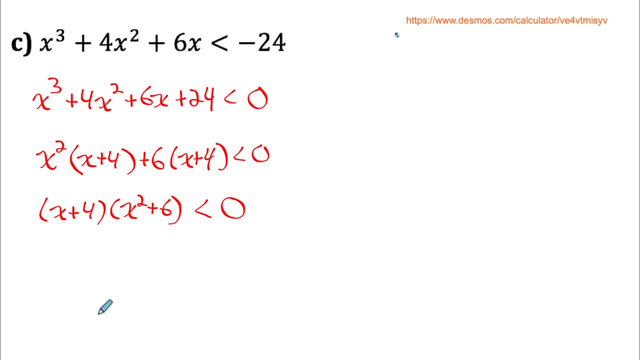 Now we have two options for how to solve this. We could solve it graphically or by a factor table. Let's just do one method for this one. Let's actually let's just do a factor table. There's actually only one x intercept here. 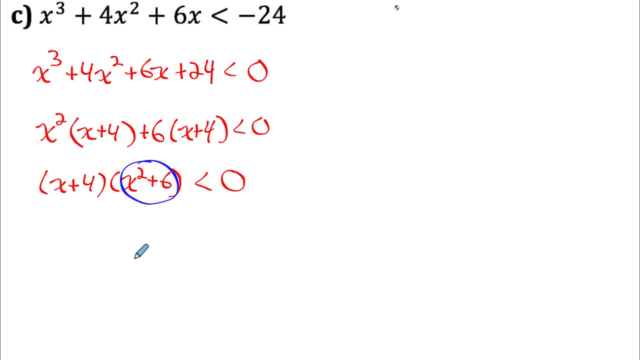 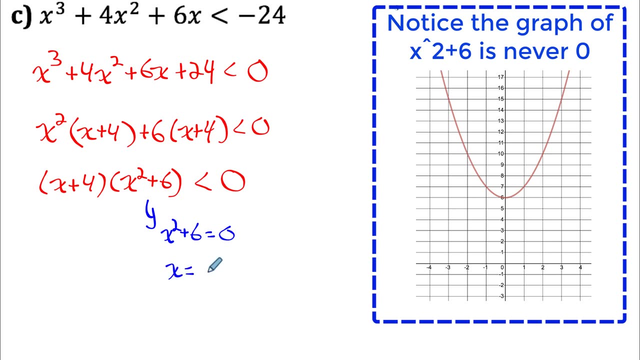 Do you see why? There's no way that that factor could be zero. If we tried to solve x squared plus six equals zero. we would do plus or minus minus the square root of negative six, And there's no real solutions to that. 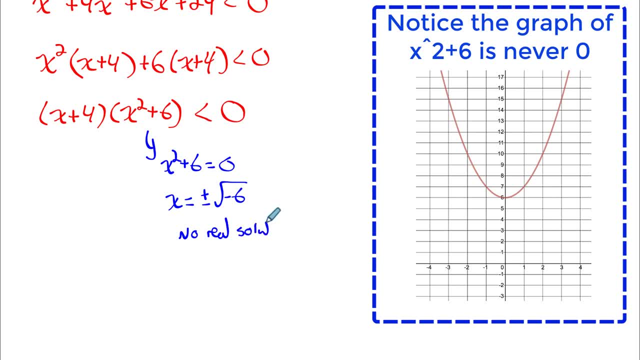 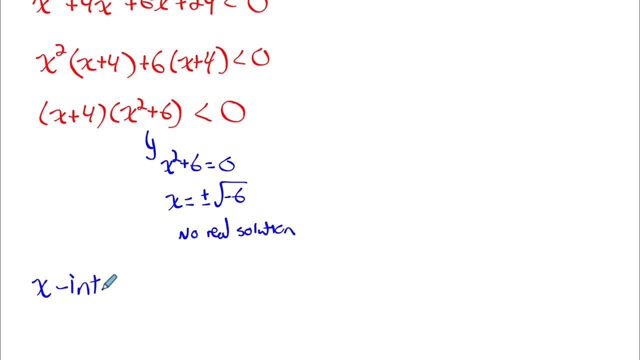 No real solution. But x plus four could be zero if x was negative four. So the only x intercept here is at negative four. So the function can only change signs, since it's a polynomial function around the x intercept. So there's really only two intervals to test here. 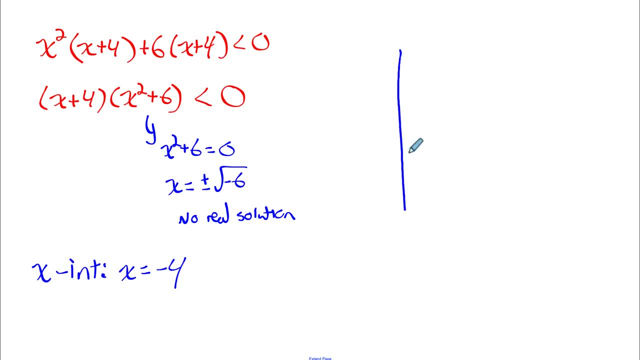 So let me make a factor table and my factor table: I need negative infinity, the x intercept, and positive infinity, And then I need a row for each of the factors. Well, there's only two factors, so I only need one, two rows. 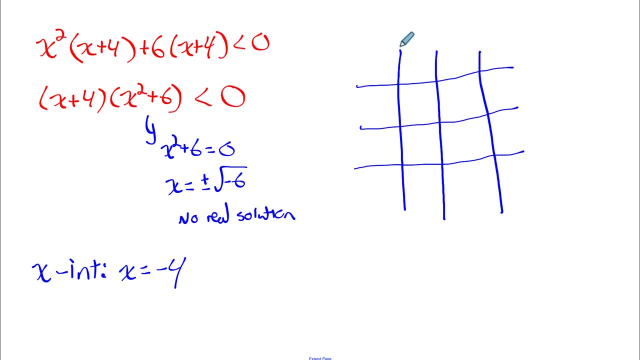 So I know this is my least organized factor table, but we'll go with it. negative infinity to infinity. And then x intercept was at negative four And my factors were x plus four And x squared plus six, And you just need to pick a test point within each interval. 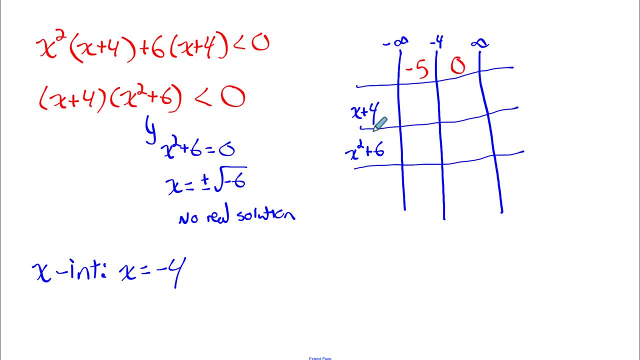 So I'll pick negative five and zero, just to make the calculations easy. Negative five into x plus four will give me negative one, and negative five and x squared plus six will give me thirty one. positive. A negative times a positive will give me a negative result. 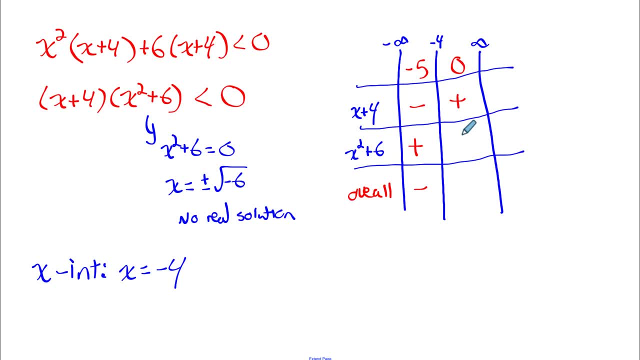 And plug zero in, I would get four and six, both positive. a positive times a positive is positive. And I want to know: when is the function less than zero? right, That's what we have here. When is it less than zero? 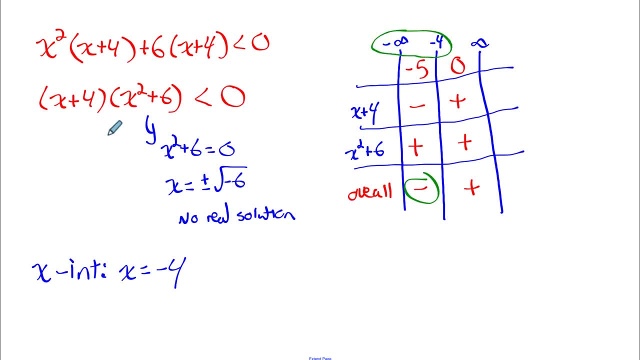 So that means: when is it negative? It's negative in the interval from negative infinity to negative four. So answer: when x is less than negative four or x is an element of numbers from negative infinity to negative four. Either way you express your answer is fine. 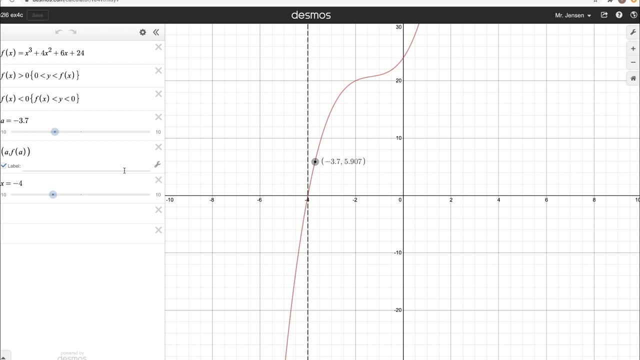 And let me just show you in Desmos to have the correct answer. Here's the function. The only x intercept is at negative four Before negative four. if we look at the y values of the points, they're negative Right. The function is below the x axis. 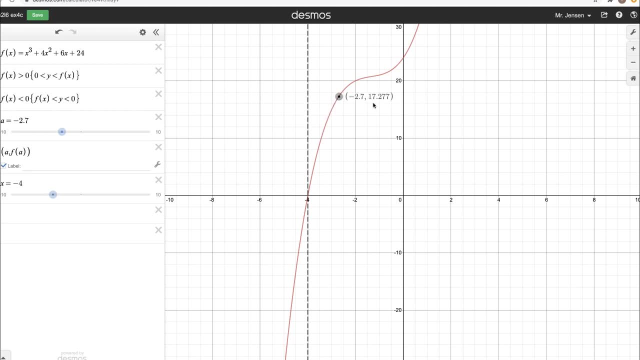 And after an x value of negative four. the function is positive, It's above the x axis And we want to know when is it less than zero? So it's less than zero in that interval. when x is less than negative four. There is an application question I have in this lesson.